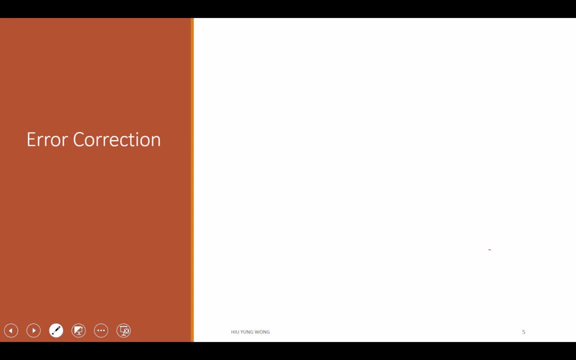 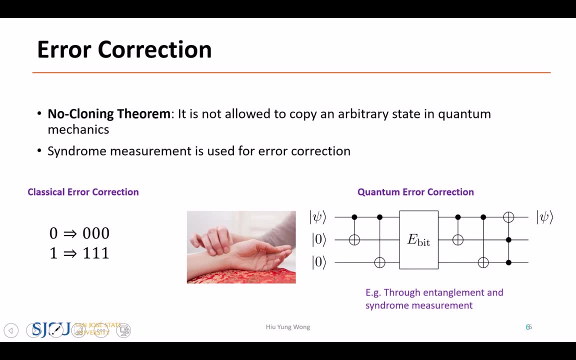 have the regenerative feature that we have in the CMOS. So error correction is very important. So let's first have an overview why there is a problem, right? So in classical error correction we use the easiest one. the simplest one might not be the most effective. one is repetition code. right, If I have zero? 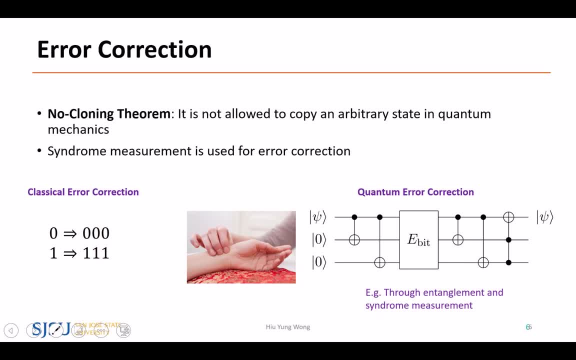 then I encode it with three bits. I have one, encode it with three bits and then if any of them got three, then I use so-called majority vote, right? This is very easy to understand. I call you on the phone, tell you the number. If it's noisy, I just keep repeating, right? I say: 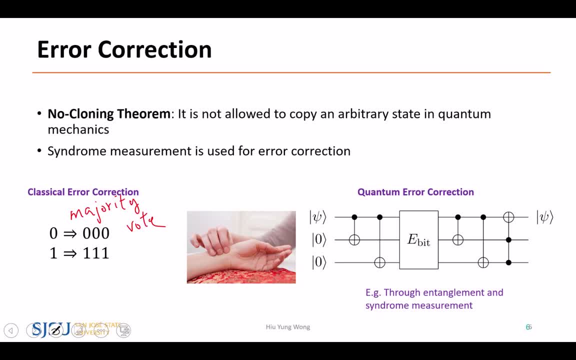 I got 100 point 100% in my exam, right? You say what? 100 or 90, right? I keep repeating. Eventually, you trust that you actually hear 100, because most of the time you hear 100, right. 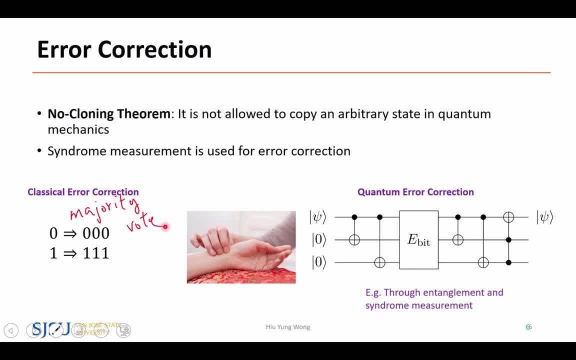 But can we do this in quantum computing? We cannot do that, because when we do this repetition it means you need to copy. We can copy the basis state, There is no problem because we can measure and copy. But for a general wave function, sine equals to alpha. 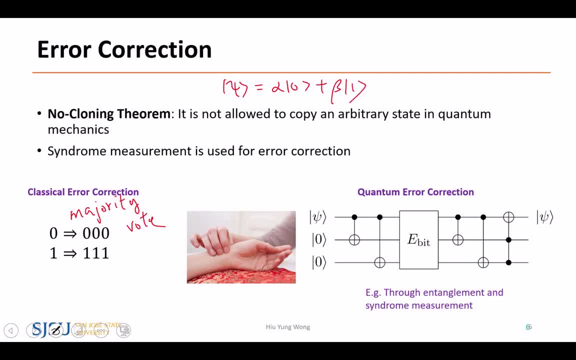 zero plus beta one. you can never copy. There's no way to copy it right. You can prove it right. There are lots of places to see how it proves, Of course I mentioned in my book also. you try to prove it. you find that it's contradictory. You can never copy an arbitrary. 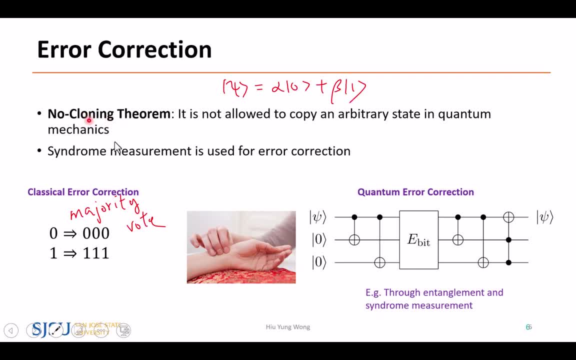 state. So this is the so-called no-Kuhling theorem, right? If you're interested, you can look at the old video in another class, E225.. Then what can we do? We actually came up with something similar to repetition code. 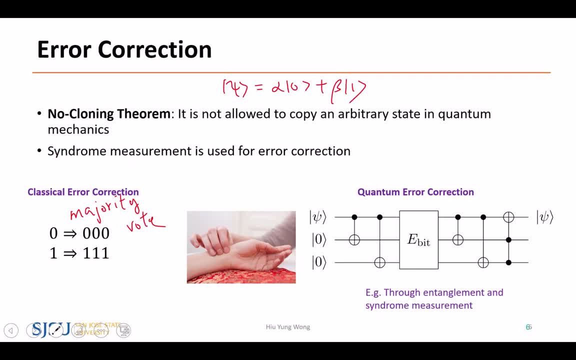 And another thing is that we use so-called syndrome measurement. So what I've seen. just like the doctor right. This might not be a very appropriate analogy, exact analogy, but just think about: if I feel that I don't feel well, I go to the doctor. I say I don't know if I have. 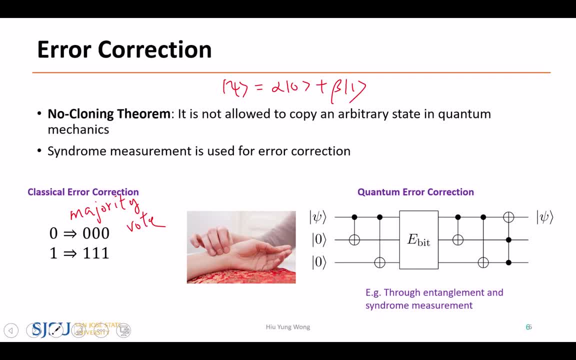 flu, regular flu or COVID? right, If the doctor is super experienced like machine learning, then he will just Just look at my syndrome, right? How often do I cough? What's the fever? How does the fever fluctuate Then? maybe without really testing myself? my blood, the virus, let's assume there's. 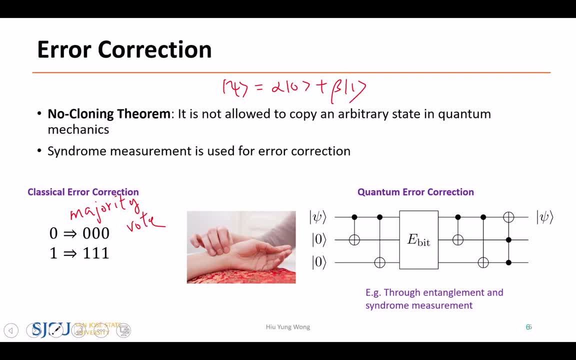 something called collapsed virus. Once you test it it will just explode and then infect everywhere in the world. So you cannot measure the virus, You cannot test it, right, You just look at the syndrome. Then maybe you know that, whether I have a regular flu or COVID right. 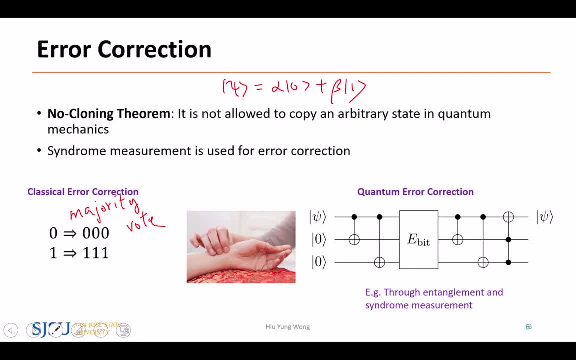 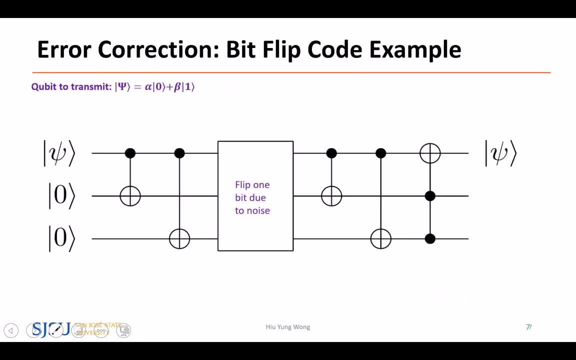 And then you apply the correct medicine to fix it. That is something like this. So in order to do this error correction, we do need to go through some entanglement. okay, So that is syndrome measurement. So this is an overview. Let's look at one particular case. This is the so-called 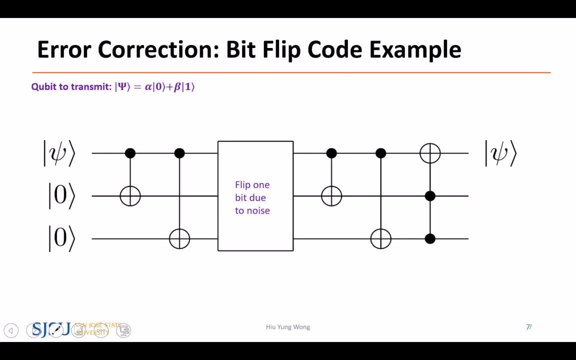 bit flip code. In this bit flip code, our goal is to transmit this alpha 0 plus beta 1.. Now we decided to entangle it with two auxiliary. Okay, these two are useless, It's not the information we want, but they're very important. 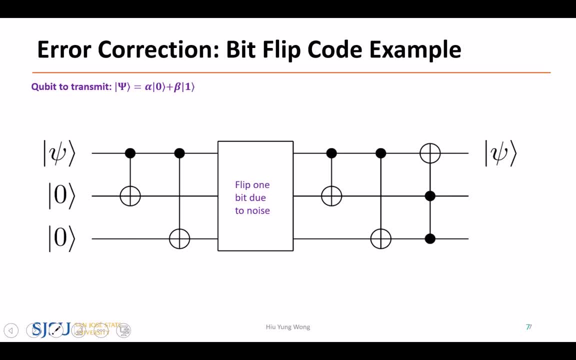 because they can help us to recover the information. So what we do is to do a knock gate, control knock gate. Now you see, control knock gate. you know it is related to entanglement, right? So what do we do? So when we start with alpha 0 plus beta 1,, 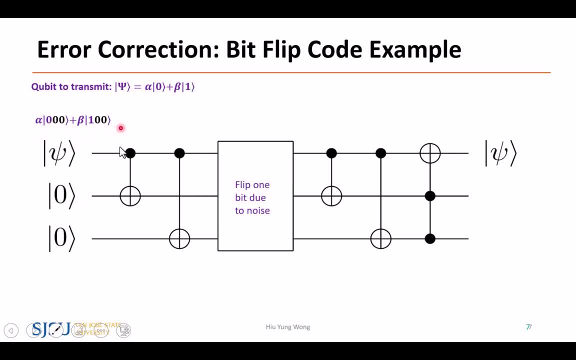 I have three qubits, So the state is 00100.. Is this okay? Everyone okay with this tensor product? right? This is very important, fundamental, cannot mess up, right? And then we apply control knock gate. What does control knock gate do? 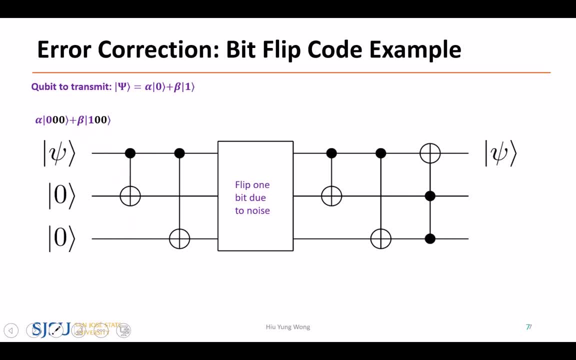 Very good. Flip the target qubit from 0 to 1, or 1 to 0 if the control qubit is 1.. Otherwise do not Nothing, Okay. so again in my hints I told you that you need to know the matrix multiplication. 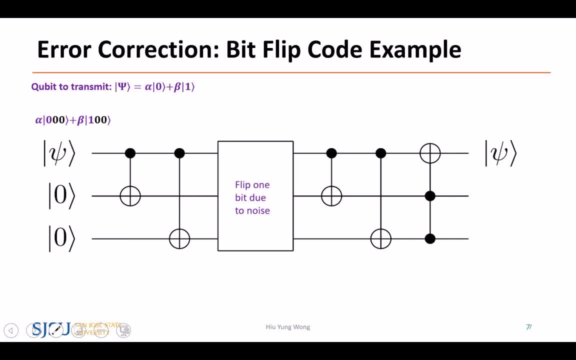 You need to do that well. So practice. I have something similar in the midterm and then we have some circuits. right Earlier in the semester we do this matrix multiplication. So this is a big hint. You need to be able to understand the circuit and how the matrix and vector evolve. Okay, 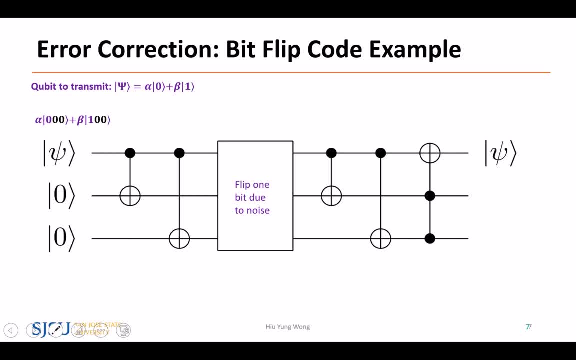 yeah, I won't tell you now, okay, But I already say matrix multiplication, Okay. so you need to have that skill. Practice the skill, okay, Make sure that you know where does the vector evolve- from left to right or right to left? I don't want you to make this mistake, right. Vector in the circuit. 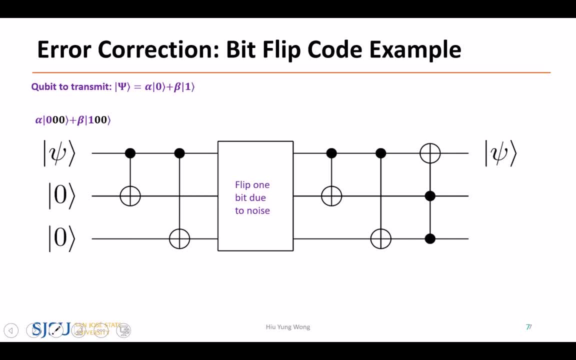 go from left to right, but in matrix multiplication you go from right to left, right. Don't make this mistake. I cannot help you if you make this mistake. okay, But here we're just using the bracket notation, We are not using the matrix multiplication. I hope that you are able to do matrix. 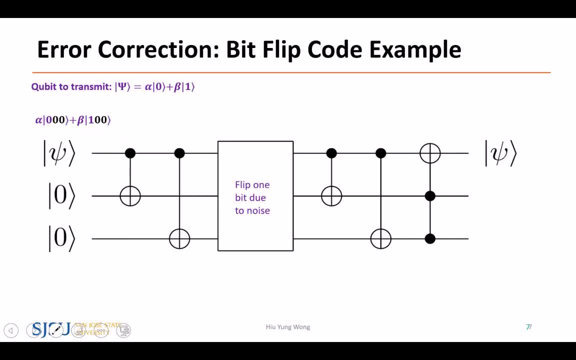 multiplication. Okay, so based on this, what will happen? Let's say, after this entanglement, what will happen? Because the control bit right, This is the control right, This is the control bit and this is the target. Both of them are the target qubit. So this is the control bit and this. 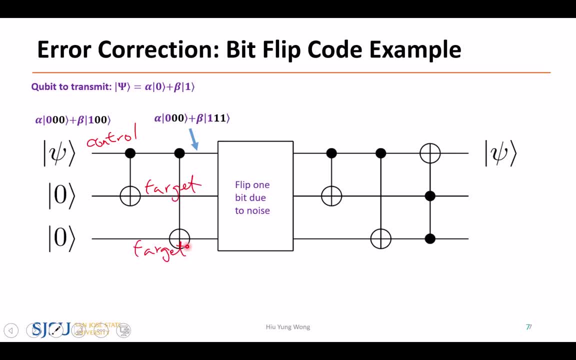 is the target qubit. What happened to this? Because it is a linear superposition, the control bit is zero, then do nothing, because this is control, not So. that's why zero, zero, zero is still zero, zero, zero, right, But one zero, zero become one, one one, and that's why this is an 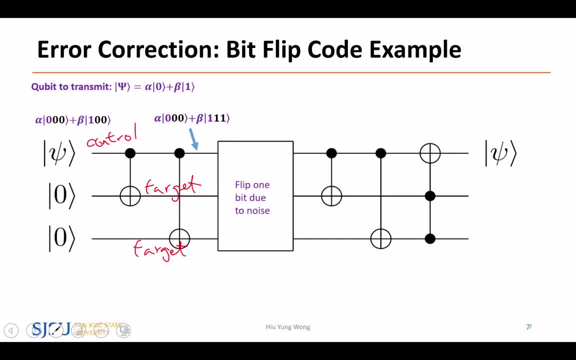 entanglement. right, This is a perfect entanglement. okay, Let's say, we go for a gate, but this is just, can be just an entanglement. So let's say, we go for a gate, but this is just, can be just an entanglement. 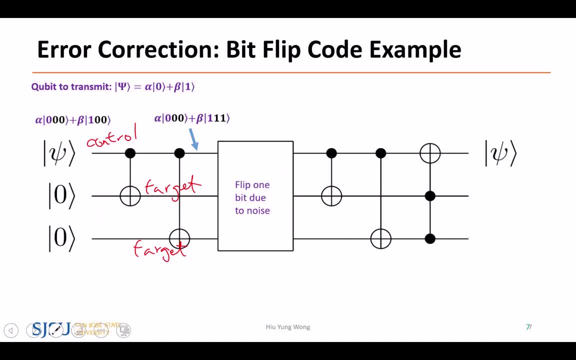 noise. It can apply to any of this qubit. Now, that is something you need to be aware of. We did not go into detail. You add more qubit to do error correction. you will bring in more error because this qubit are not going to be perfect, So you need to have a small enough error rate, or high. 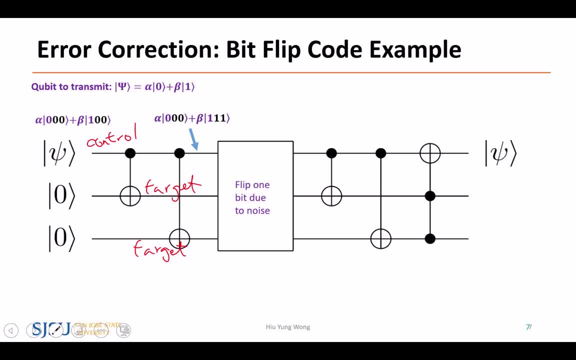 enough fidelity for your physical qubit in order to add more qubit, right? So that is the challenge that you need to face. So let's say: you have a gate and you have a control bit and you have a keep the balance. okay, So let's go back to here. Let's say, very unluckily, we flip the first qubit. 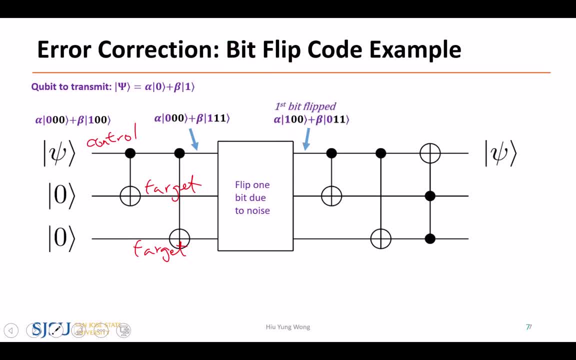 That's why this is a bit flip code right. We only deal with the flipping of the qubit, Then the first qubit. when you say you flip a qubit, basically say you apply a, not gate, to it, right, For example? 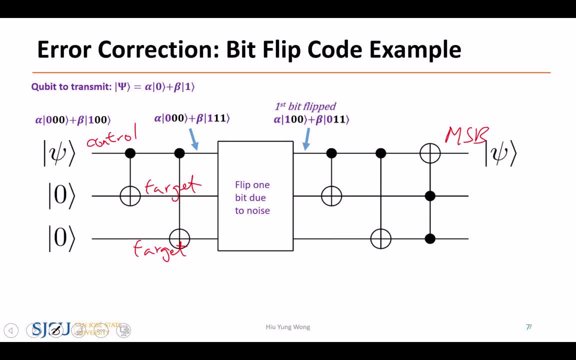 this is like what. If this is the MSB right LSB, You understand what is MSB and LSB? well, right, Then this operation is going to be like this. So this is going to be like this, So this is going to be. 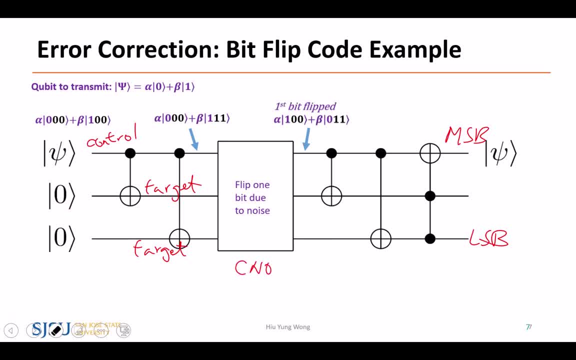 like this: So this operation is just what C is, what Can you tell me What would be the operation for changing from here to here, Not gate for MSB, and then how will you write it? I want to apply the free qubit. Yeah, so then the tensor with: I. 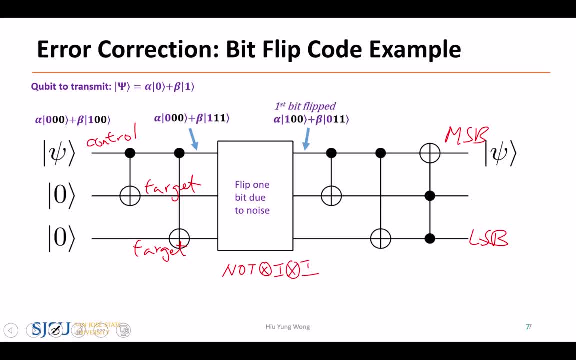 Tensor with I: Yeah, right, This is a basic thing, right? If you cannot do this basic thing, you cannot do the exam. okay, If you don't understand practice, Okay. so I flip this one, right? So in principle, I can write this in vector form. I write the: 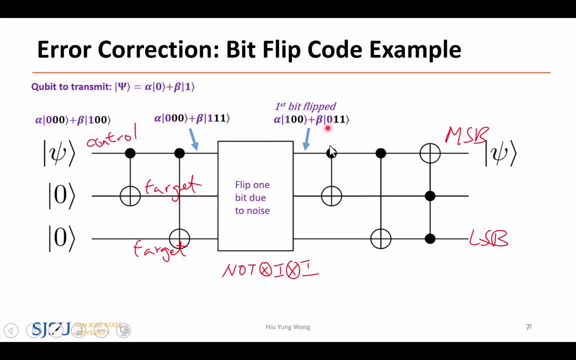 matrix. I will get this also. okay, Okay, that's okay. Now get got flip. We cannot measure it because it's quantum state. So what do we do? We entangle this one more time. What will happen when we entangle it? When this is one, then I'm going to flip the second bit, and then next time. 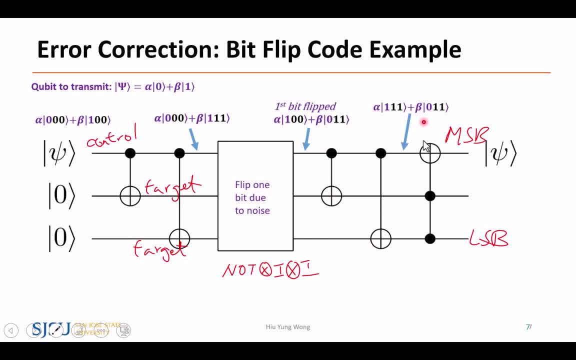 flip the third bit. So I get one one one, correct, Because the first time I get one one, zero, The second time I get one one one. The first one is zero, I do nothing, okay. And then 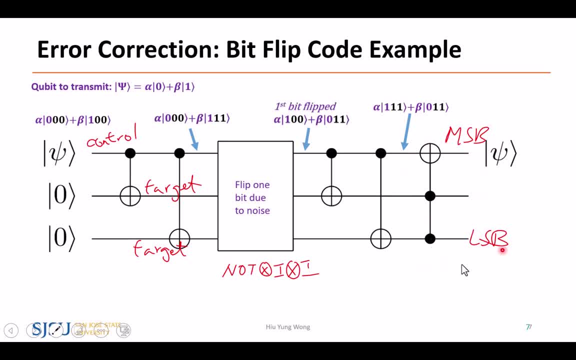 I have this automatic correction at the end, which is reverse. This is what type of gate, Do you know? Did I mention this Portfolio gate Control control not. Maybe I did not mention at the beginning, but this is control control not, Which means if both of them are one, I'm going to flip it. 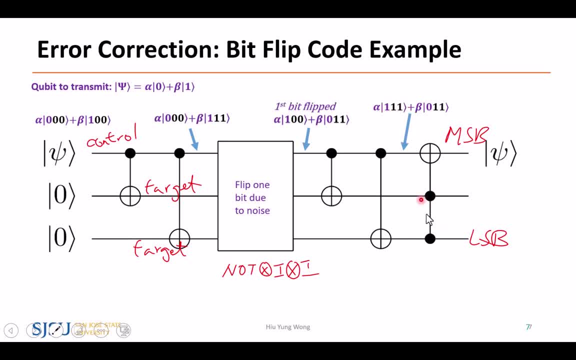 and then I'm going to flip this. The last two bits right is one one, right, Because they are LSB, Then I'm going to flip this to zero one one. These two are one one, right? Then I'm going to flip it. 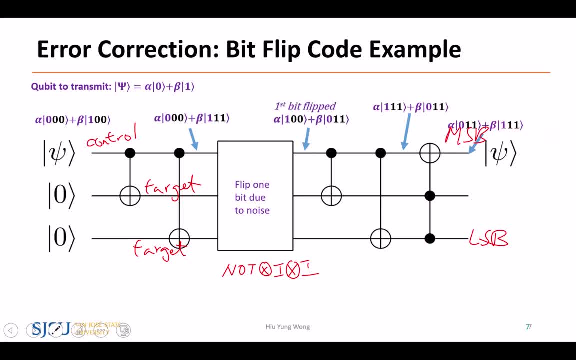 become one one one, okay. So in this whole process again, these two are not entangled. now I can take these two out. This got corrupted, but I still get alpha zero plus beta one. okay, Yeah, Will this work if they're only flips? 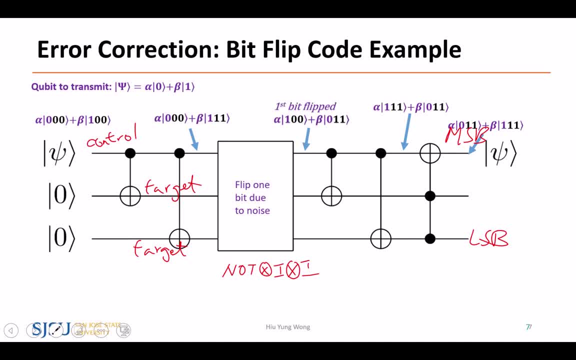 Yeah, that's the problem. Nope, If ancilla flip, there's no problem. You just go through this. I have this here. Go back to practice. but only one qubit. If you have two qubit flip at the same time, then this doesn't. 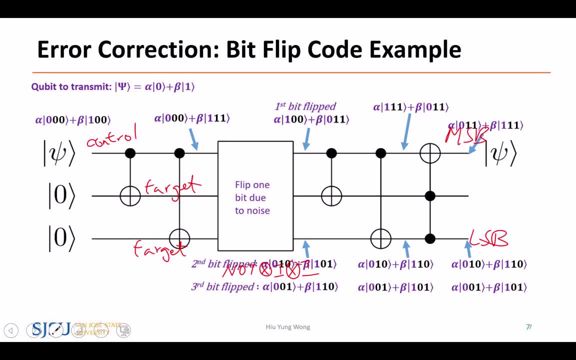 work, okay, But of course then we will start saying: let me erase this over there. You know what I mean, right, It's not The probability of getting one qubit flip may be p, another qubit may be p squared, so this can be pretty low, right? So you need to improve the. 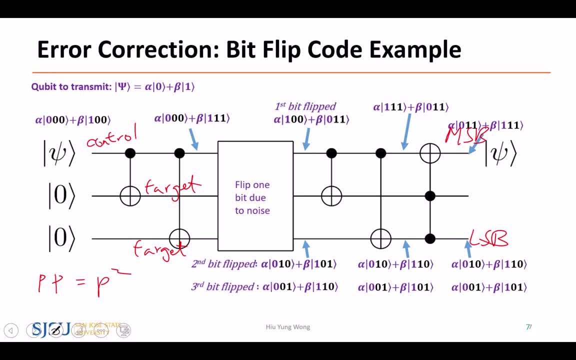 technology until the p squared is low enough. if you want, you just want to use this. okay, Good, So any questions? Yeah, So I guess to build the recurrence you need multi-bit entanglement, isn't it? You need to? so let's say, yeah, here you have three qubit entanglement. 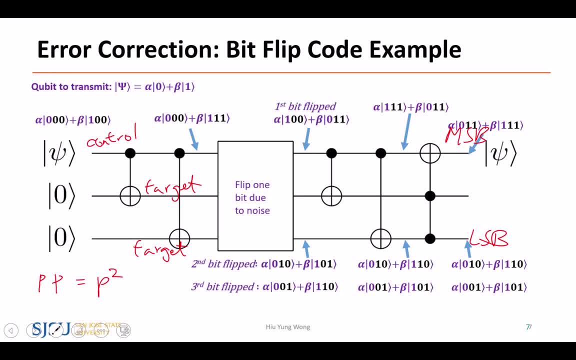 So let's say four, Five, Yeah, this is just a simple example. Yes, you only entangle all of them, but this is just simple example. You use three qubit, right? Let's look at another example. You may say: how about you? 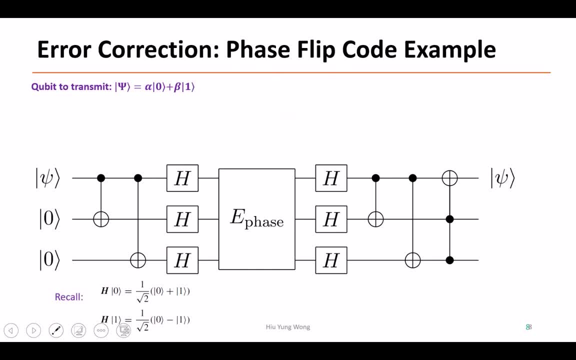 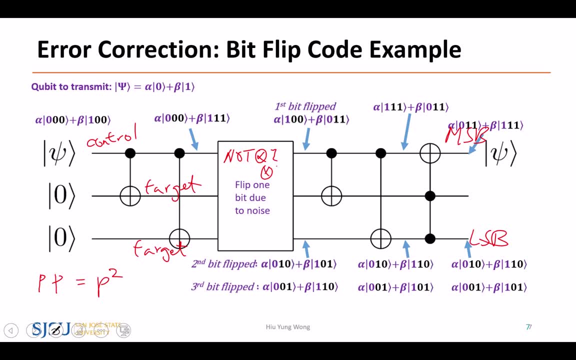 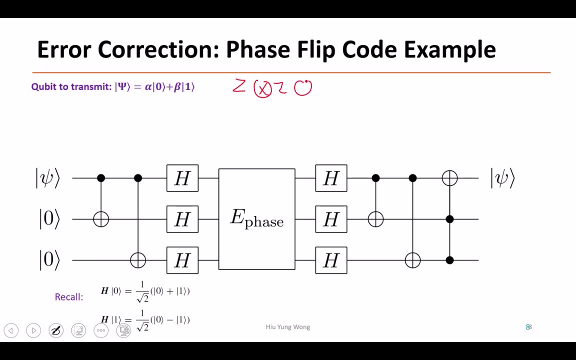 have a phase flip, Phase flip. basically, here I use not tensor product, i tensor product, i right. What if I have something called z tensor product, i tensor product, i okay. This is related to maybe p2, right. So what do we do? Now it turns out that 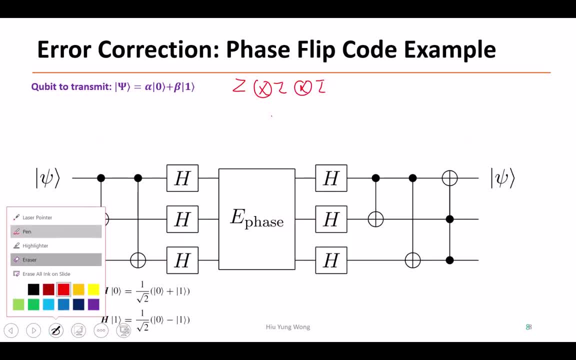 this is also easy. What we are going to do is treat it as a bit flip. okay, But then if we add the Hadamard gate to it, it's equivalent to the phase flip. So we are going to do a phase flip. 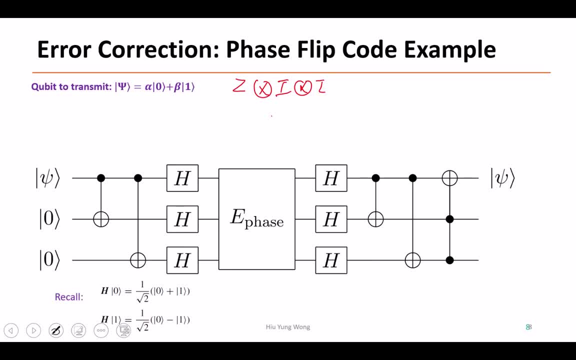 okay, Because h equal to z. Am I right in this one? I think so, right. So the phase flip is just a bit flip. So what we're really doing here is this. I first entangle here. let me see if I have. 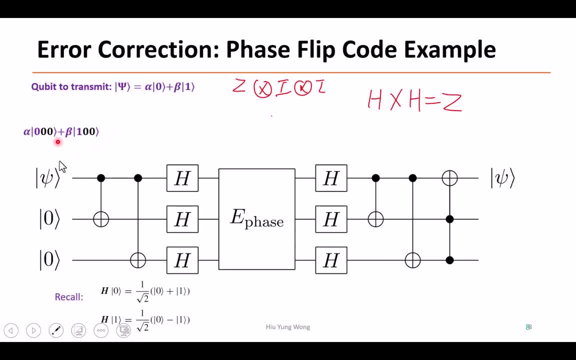 anything. Yeah, I start with this one. this is the information I want. Again, I do entanglement, So I have 000111.. Now I can analyze the phase flip by assuming the whole thing is just a knot gate, and then with the Hadamard gate, 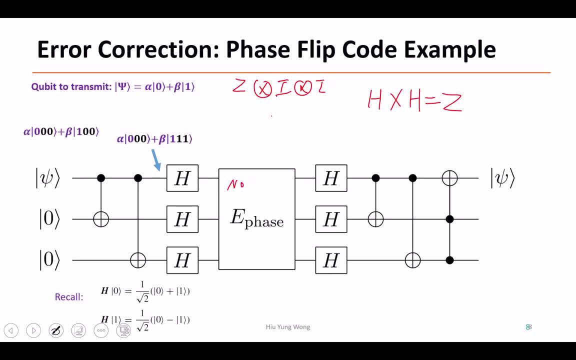 This whole thing right. if I put this as knot, this is just a modeling of the error- Then this whole thing is just equal to this one. okay, Why is that? Because the Hadamard gate is going to change my zero to plus. Remember this Hadamard gate. 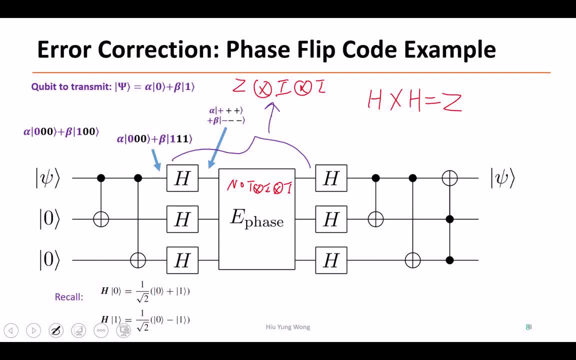 abide to zero, it will be superposition right, which is plus, and then this is minus. okay, yeah, What do you mean by both Hadamard gate and the Hadamard gate? The line be closed the first time, but not the second time after the phase flip. 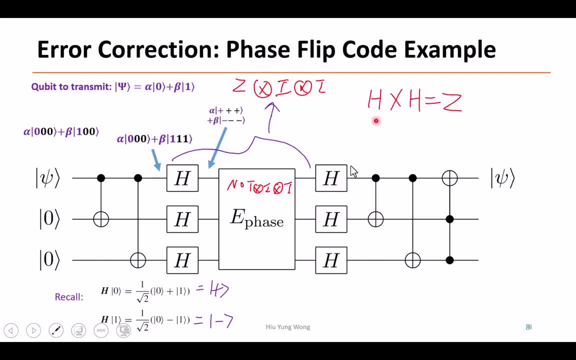 What? my line This is H and then X and then H, So that should be equivalent to That, equivalent to Z. yeah, Okay, so I here just go through the math, right, and then you have a bit flip, right, because after 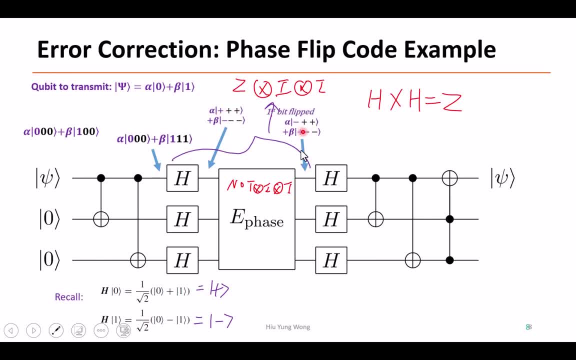 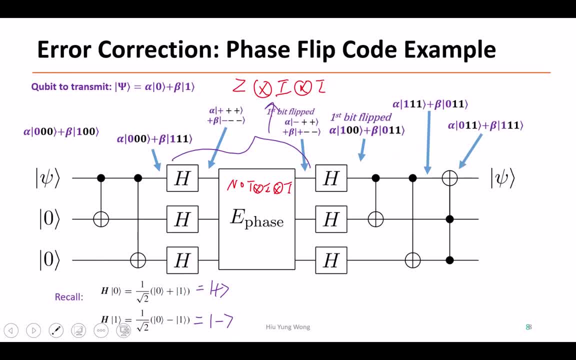 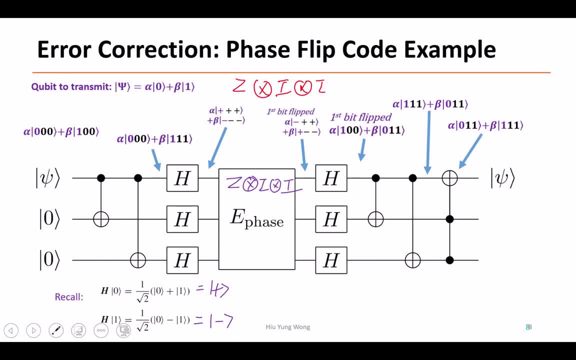 h x h. that would be just for the first qubit up there. yeah, right, so if you just replace that block, you can replace that with h x h within that block, just for the first, the first. indeed, yes, in this particular case, right, because i only flip here. right, so this is equivalent to: 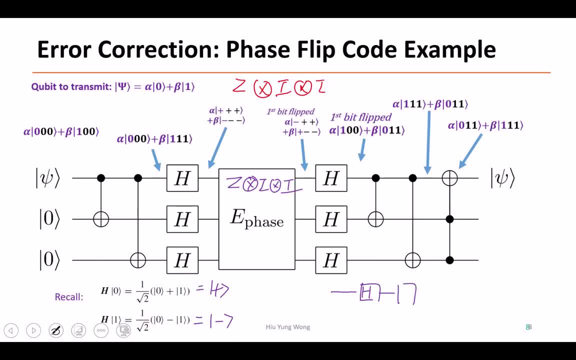 this: h, x, h, h, i pressure- and then h, i h, where extra h, this is h, and then x, and then h, this is h. huh, you know right, uh, z, c, c, sorry, sorry, yes, my question is replace that z with conditional age gates and within those. 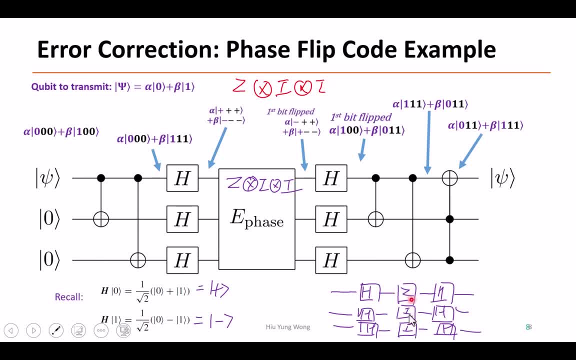 age gates. no, the point is this: z is given by the noise. you cannot control it, right? yeah, so this is just z. well, yeah, because i was asking, did you put it equally? so i was saying equal to z. you should be able to replace z with h, x. 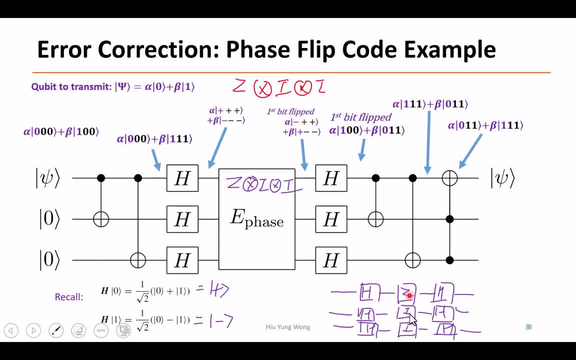 h. remember, you mean this one replaced by h. yeah, you can do that. yeah, yeah, for your analysis. but the noise actually come from as z, right, because that is the environment noise. that did the phase flip for you. so it is z. yeah, you can put h, uh, h, x, h then become x, right, that is. 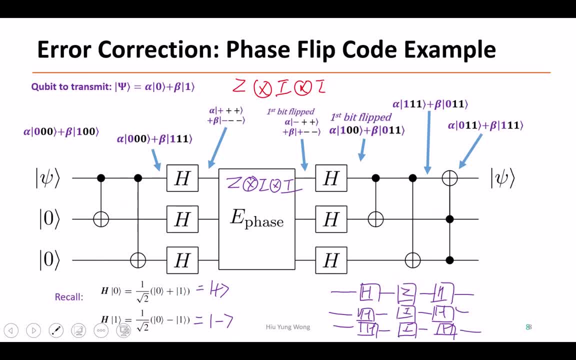 why the rest? i can treat it as a bit flip. yeah, do we often see, you can see it. it can be a bit flip, but you can see it. Do we often see like full bit flips in quantum computers? It seems like most of the way we implement our gates. 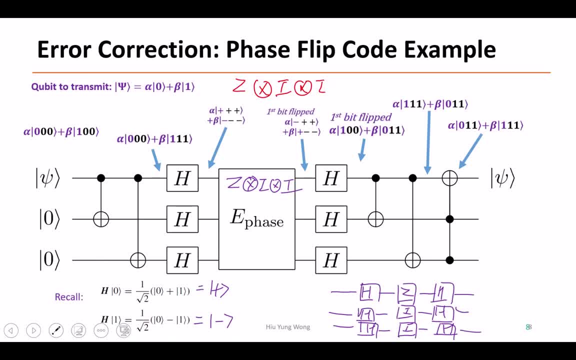 is by like doing a timed pulse. So I would imagine, like what more likely is that it's just like slightly off rather than a full flip. Yeah, I don't know this well, but the point is that I'm going to talk about this. 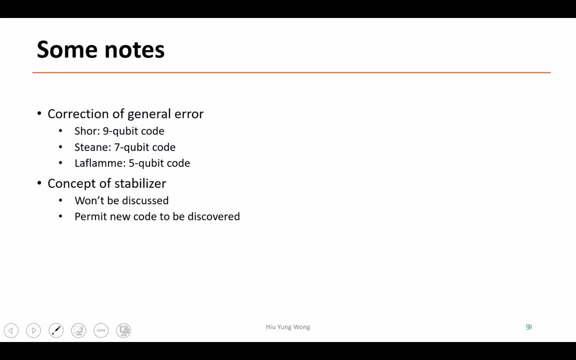 In general, if you have this bit flip gate and the phase flip gate, you can do the correction of anything. Yeah, it just mathematically show that. Yeah, I did not go into the detail, So, yeah, that is something you have a great question. 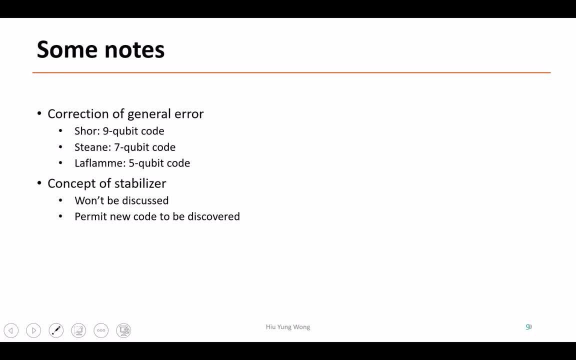 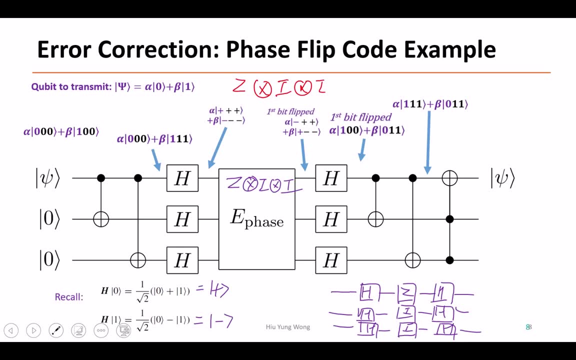 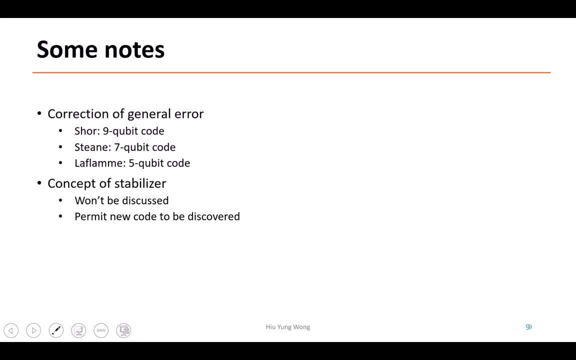 and I was not able to really answer you, but just this tool will be enough to make the correction. So then, how do we correct both the phase flip and the bit flip? You have the so-called short nine cubic code, So you encode with nine cubic gate for one qubit. 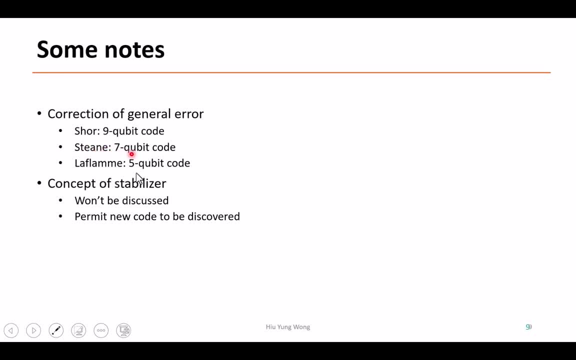 to do this correction. But then people have been improving. The smallest one is five qubit. They are able to do five qubit encoding and then can flip both the phase and also the bit flip. Okay, just for you to know right. 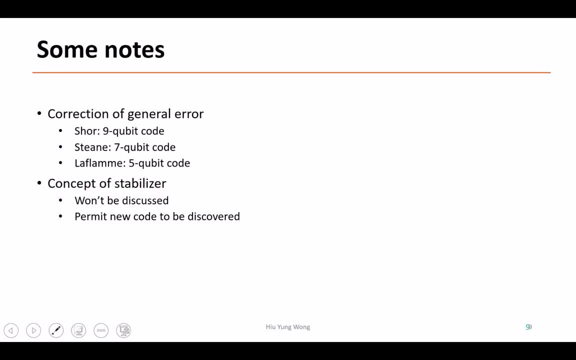 There's something I encourage you to study later is the so-called stabilizer. This concept is very useful. Based on this, you will be able to discover new code, right Because when Shaw invented this, just because he's smart, and come up with this algorithm. 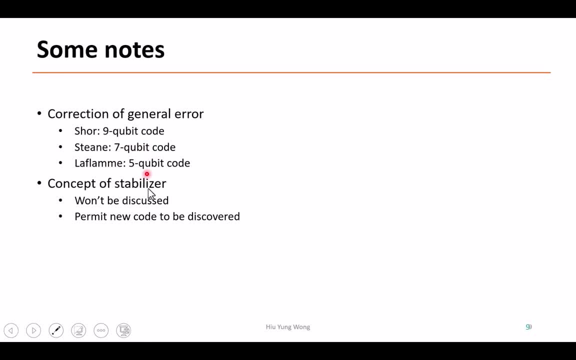 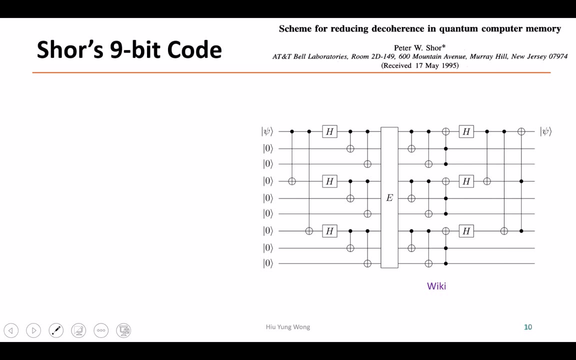 But if you want to continue to derive something not that intuitive, then you need to understand the concept of stabilizer So you can think about that. So the last topic I want to talk about is the Shaw's nine qubit code. Okay, it has quite some math. 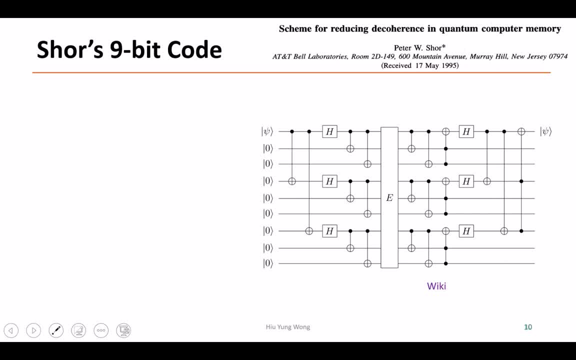 but it helped us to understand the things deeper. So what is that? So the goal is this: I have the zero state I'm going to encode. This is encoding with nine qubit gates in this way: One over square root, two zero, zero, zero plus one, one one. 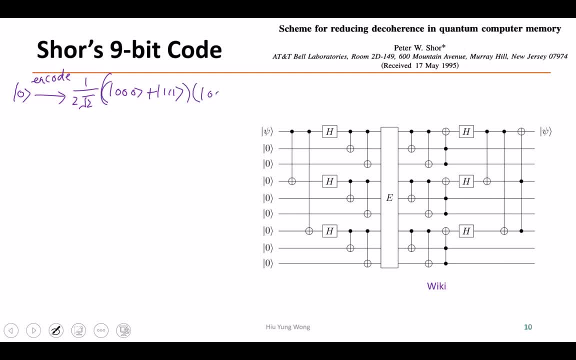 And then I'm going to do it three times. It's like this: And then I'm going to do it three times. Is that correct? Yeah, This is. I hope that you understand what I'm talking about. How many qubit do we have here, based on what I'm writing? 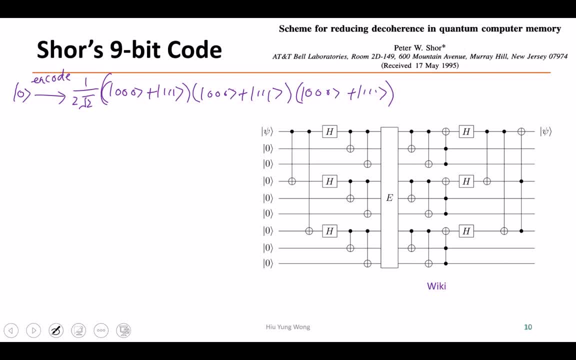 Nine, Nine qubit, Do you agree? Yeah, Okay, so I have nine qubit. And here I have. how many qubit? Nine qubit, Okay, All right. And now let me see. And then here I learn about the faktiskt product products. 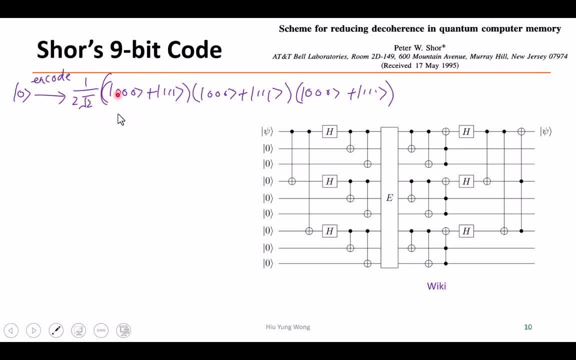 I have a lot of products in here, So I have nine qubit, 3 qubits and they in a superposition of two basis state: 000 and 111. okay, so this one I definitely can write it as 1 over 2 square root, 2 000 plus 111, and 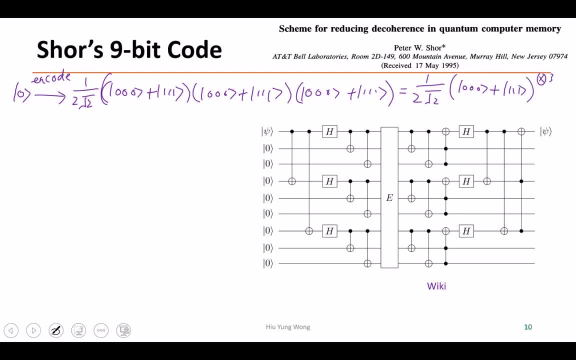 then three of them right tensor product. so I, if you're I have a 0, I will encode it by 9 qubits in this way. okay, and then if I have 1, then how do I encode it? I'm good to encode in this way 000 minus 111, and then again I'll repeat. 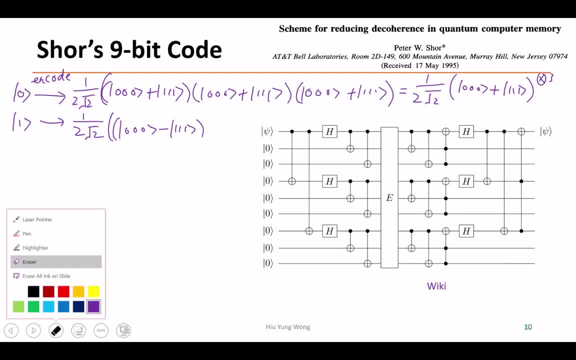 it for 3 of them. maybe to save the space, I just write this. I hope that you understand what I mean. now, right, 9 qubits, three groups, three tensor products of the tensor product of three subspace. each subspace has three qubits. right and the 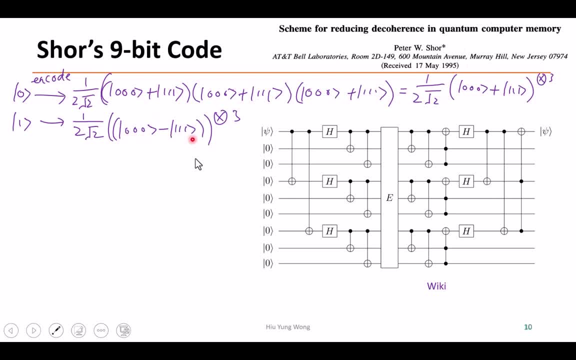 code is zero, zero, zero minus one, one, one again. linear superposition of two basis states, right. so then, what does it mean? that it means we will transform this to this right, and maybe I should- sorry, I should- make it clear, then we call this one zero. let me call it. 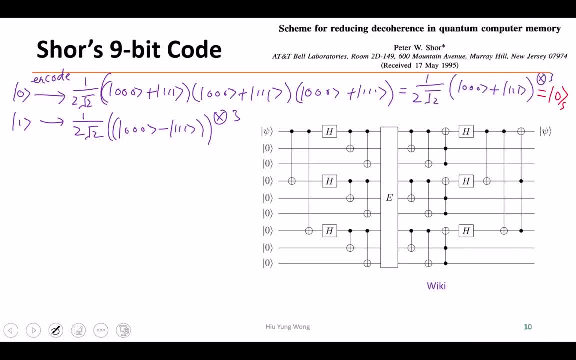 zero s right, the encoding one one s right. when I say one is no longer one qubit, just a notation, okay, it means nine qubit. this is the encoded one and encoded zero right. so basically we are saying that if I have alpha or the psi, I'm showing in this figure psi. 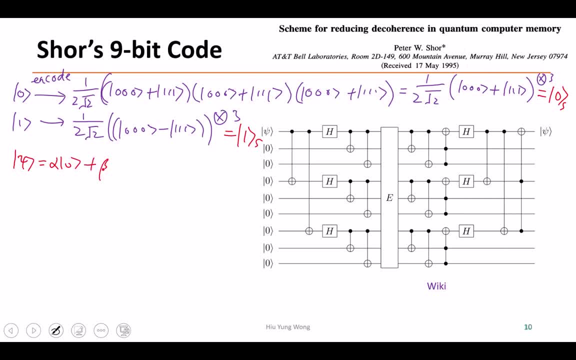 equals to alpha zero plus beta one. I encode it as alpha zero s plus beta one s. is that okay? okay, let's say, unfortunately I have some error. so where one is the meaning of error, any quantum state. it should not lose its information because everything is quantum. 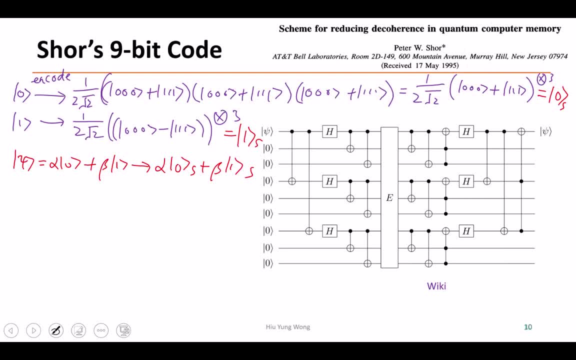 the reason that it lose information, because it need the information to the environment. it entangle with the environment, right? so we might have an environment state originally, right originally. or maybe I say with the environment, I call it e zero, right, so the original state is what e zero? 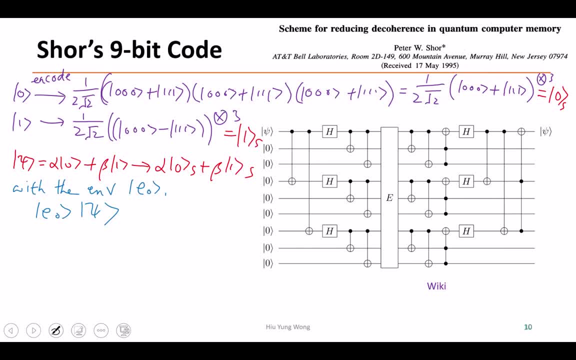 psi, are you okay with what I'm writing? I encode the environment state and combine it with the qubit state. I'm interested in again that tensor product right, you can even think, or maybe this another qubit and you don't want it. it's just an environment whatever. 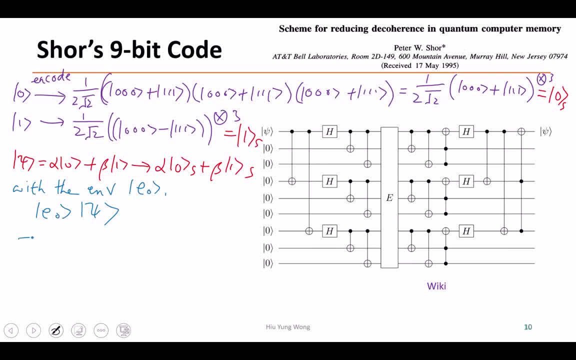 right then what happen? it transform to what? this is equal to alpha e zero zero plus beta e zero one. however, I encode it already. I assume I already encode it. right then it that means it has nine qubits. okay, it becomes this, okay, so I assume that. 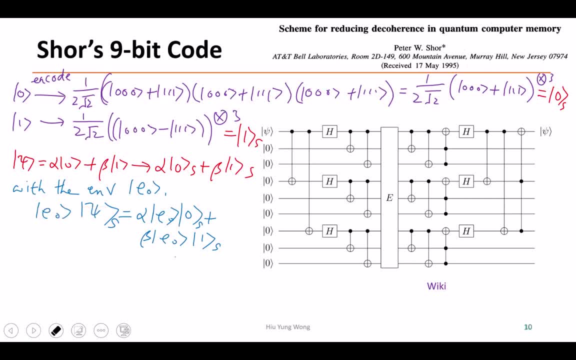 due to error, and this error come from the environment because it entangle with the environment. right, if the environment has no effect on the qubit, if the environment has no effect on the qubit, then it will just keep as this. right, and I discard the environment, I get back my side. 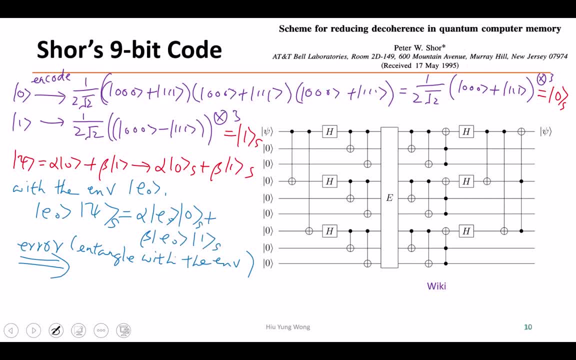 because they are not entangled. but now let's say somehow they got entangled. then I will do it one by one. e zero, the e zero, the e zero stage with zero s maybe becomes a zero zero plus a one one. this is very general, that will answer. 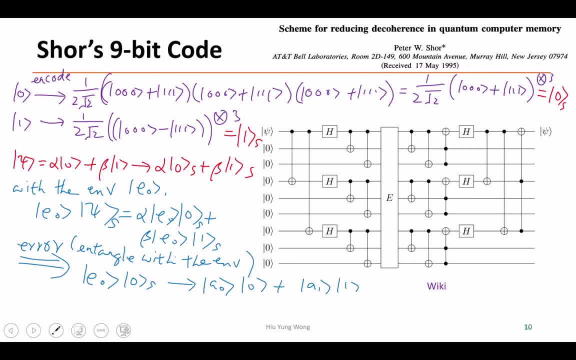 your question right. the rotation is not bit flip or phase flip, right. it's just any possibility, because I can have any combination with a zero. a zero and a one can be anything that it means my, and then if you look at your qubit right, it becomes a very 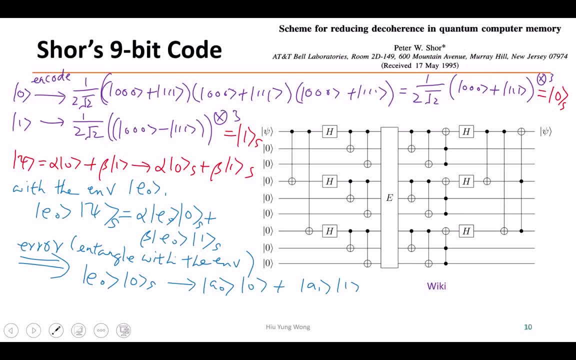 general possible state. yeah, at what point on the circuit is this red state? because it's initialized. the red state here is here. oh, I think it is here. I think so. yeah, I did not check, but I think so. okay, maybe you can try to check. it's here, yeah. 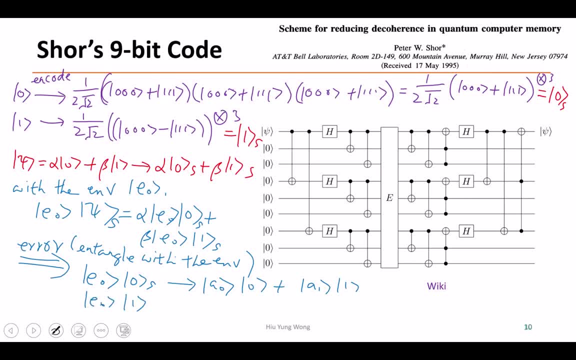 now, then I also assume e zero of this guy becomes a zero plus a three one. okay, just it. I have this super. just have this error entanglement, right? so this is just an entanglement. entanglement with the environment. okay, and I'm going to consider them. 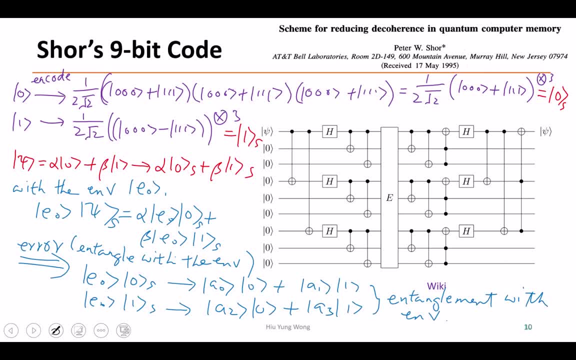 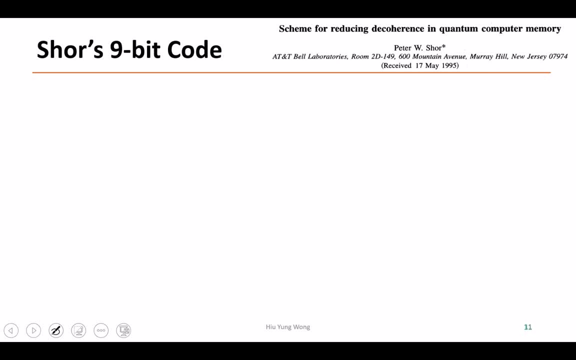 separately, because it is linear. okay, so let's look at this. what I'm trying to do is just rewrite what I had right, so now I just rewrite the whole thing. we have e zero. originally it is alpha zero s nine qubit one s right. this is before the error. 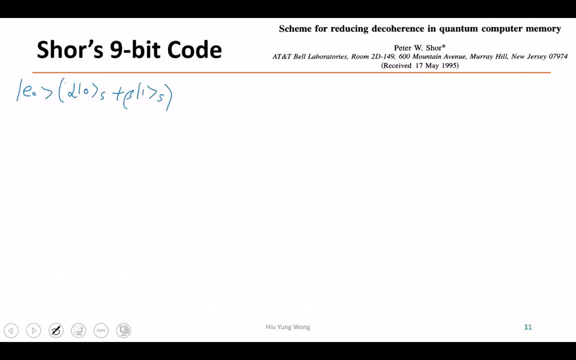 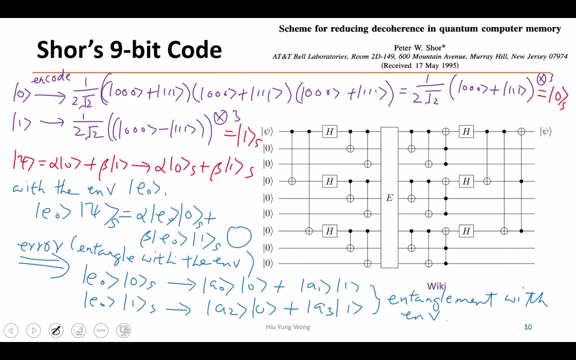 this one, right? I'm trying to write it again and now I will spell it out. this one equal to what? equals to e? zero, two square root two. maybe for your study, let me call this equation one, right? so actually I'm just repeating equation one, okay, so what? 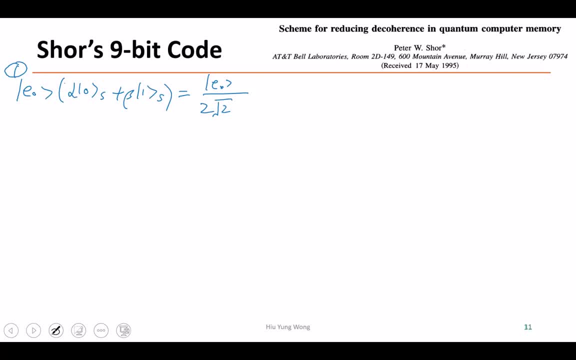 is this alpha? zero, it is alpha. do you remember how we encode zero? thank you. zero, zero plus one, one one. but you have three qubit. yeah, you have nine qubit. and then plus beta, zero, zero, zero minus one, one one, which is the encoding for one right. 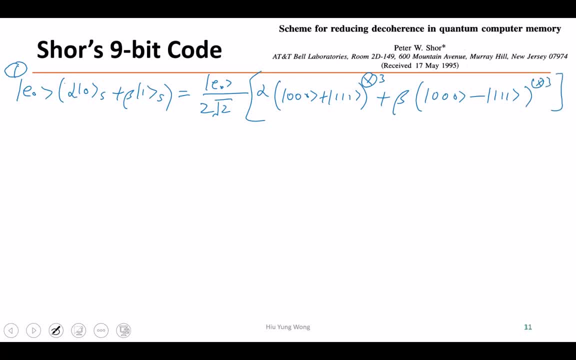 and again. do this right now to simplify, right I, since the last six qubit are not entangled. right, because we assume- here I only give you one, one of the possibility- that because we assume the first qubit has error, right, we keep only assuming only one qubit. we have nine. 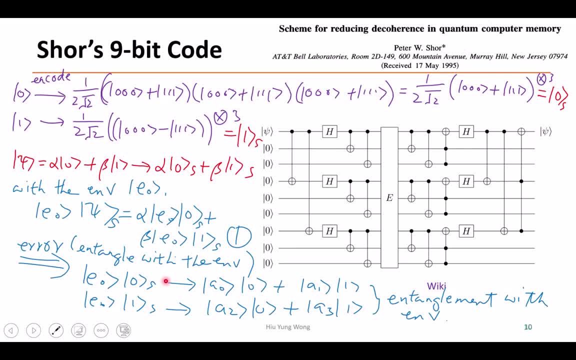 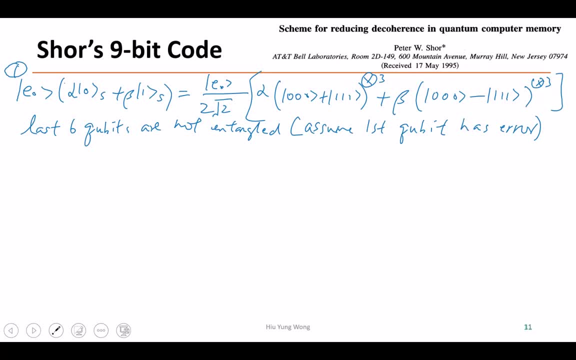 qubit. we assume the first qubit has error, like what we're showing here. only the first qubit has error, then I will just ignore the last three, the last six, just to ignore them in my derivation, right? so ignore last six for simplicity. okay, so so with. 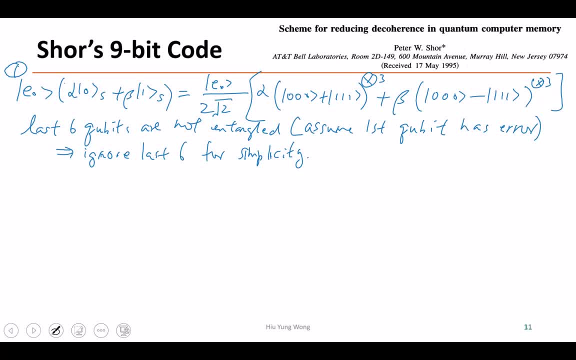 how many pages? so with this? then I have this. the first one is again E, zero divided by square root two, and then times alpha: zero, zero, zero, plus one, one, one, and then this is for this one. okay, that's the first term, right? and then of course the 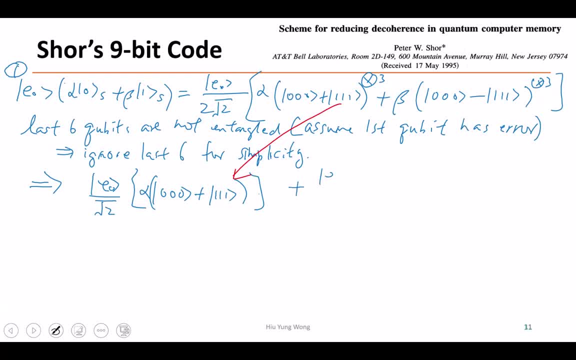 whole thing is going to be: plus E, zero, divided by square root, two beta zero, zero zero minus one, one one. so I did not do anything new, right? what I'm doing is just ignore the last few qubit and then rewrite this equation before having error. that is how you. 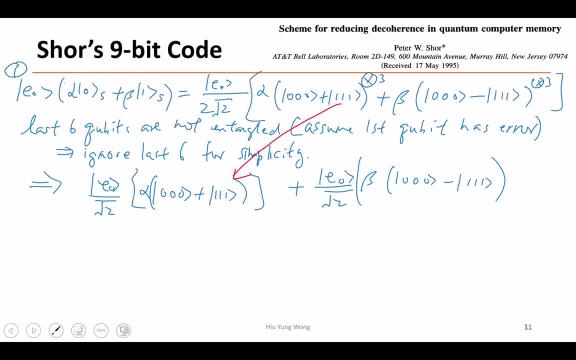 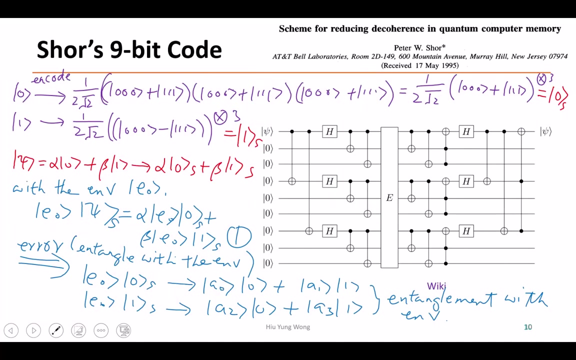 entangle with the how you, when I combine the environment and this one right now, and then when there is an error on the first bit, when there's an error on the first qubit, then I'll just repeat here, repeat what I say here: this E zero applied to one. 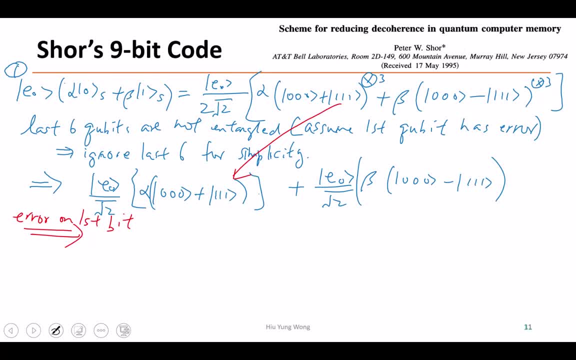 is going to give me this. actually, I need to do it one by one, right? I will go this one first. okay, when E zero applied to alpha, what do we get? I take this out: alpha divided by square root two- this is alpha divided by square root- and then E zero applied to. 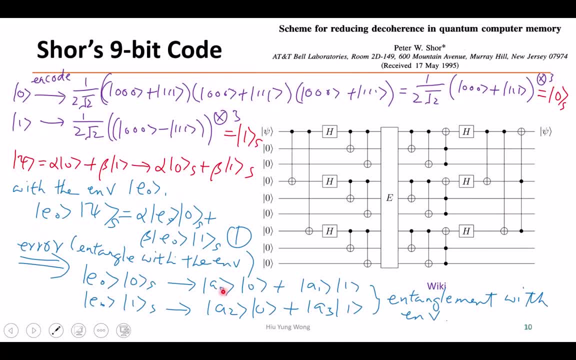 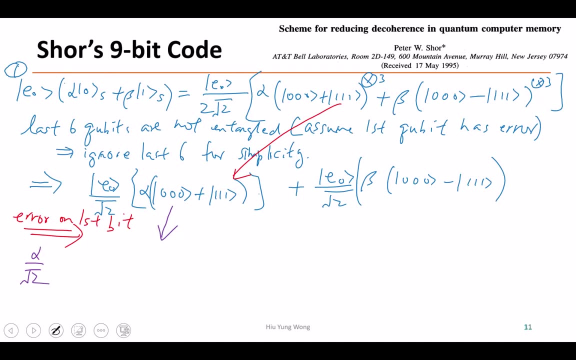 zero right. E zero applied to zero is becomes A zero, zero A one one actually. I. now I realize I should not put this S, because I only wanted to talk about one bit. the error come to one bit right, so it becomes: when this is zero I have. 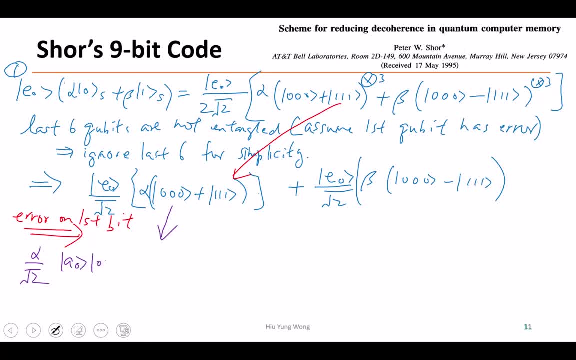 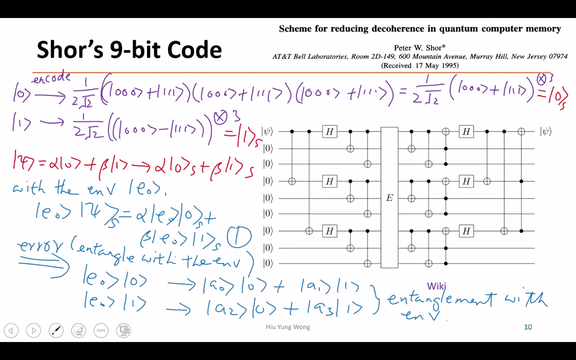 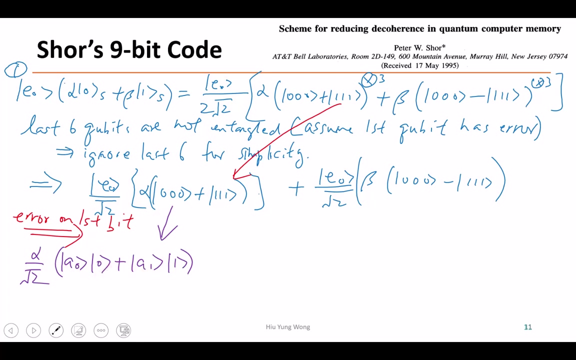 A zero, zero, zero, zero, right. plus maybe I factorize it, then it will be better- plus A one one. the whole thing right. why this? because this E zero zero become A zero, zero and A one one. so this is: E zero, zero become A zero, zero and A one one right. 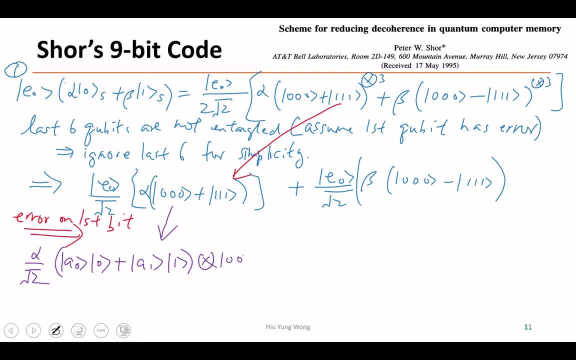 this whole thing. tensor product with zero. zero plus A two, zero plus A three: one. tensor product of one one. do you see that? because this only apply to the first cube bit, to the last two cube bit, I keep it as it is: zero, zero is still zero, zero. 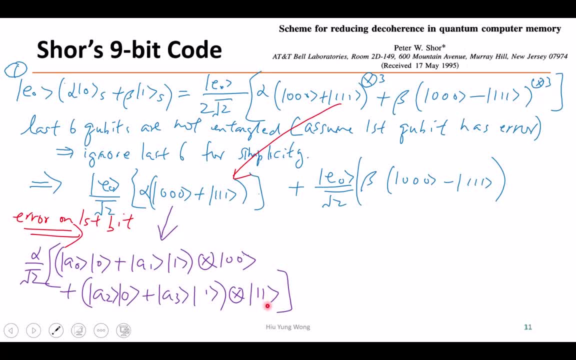 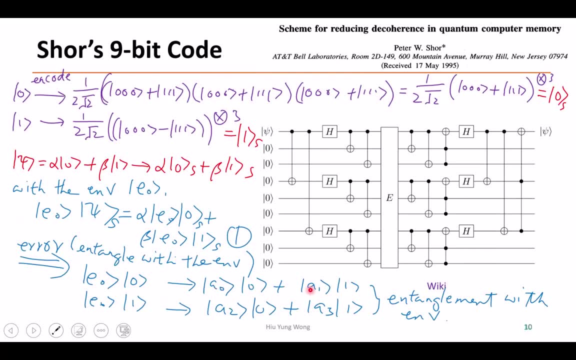 one one is still one one. but I then have E zero to zero. right, E zero to zero, as I show you, becomes A zero zero, A one one, it's just that a general state. and E zero one becomes A two zero and A three one. that's what we. 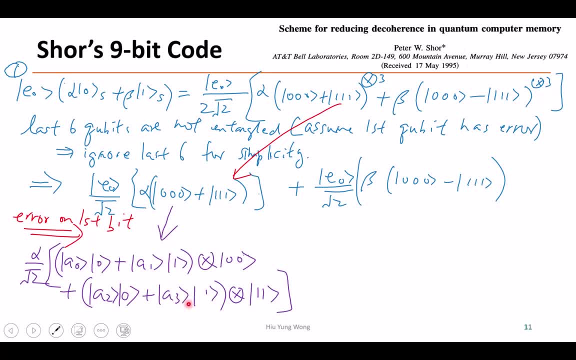 will have here. okay, so this is the state that we have. okay, how about for this one? we have similar thing. we have beta divided by square root. two: let me test if you all understand what will be the first item when I apply beta, I mean when I have error. 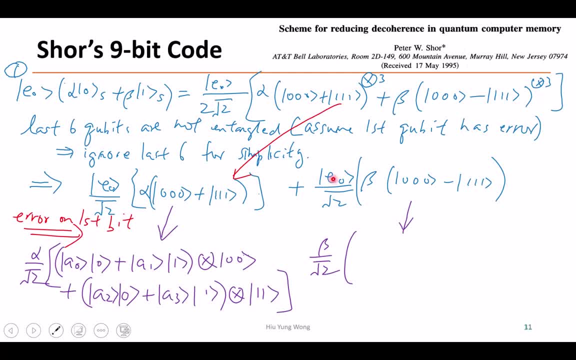 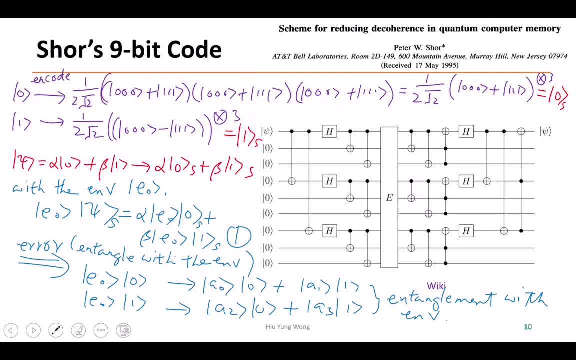 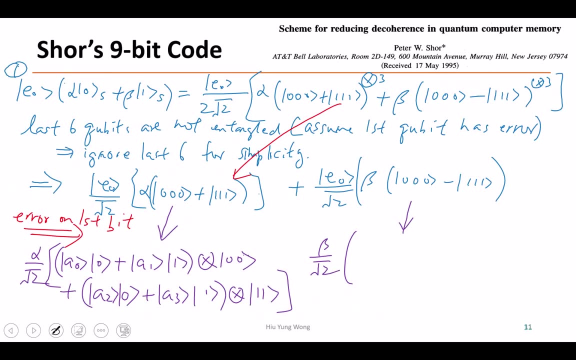 E zero zero becomes what right this? E zero zero together. when I have error, flip the first bit. it becomes what? it becomes A zero zero plus A one one, right. so it is the same it is. it becomes A zero zero plus A one one. the whole thing. 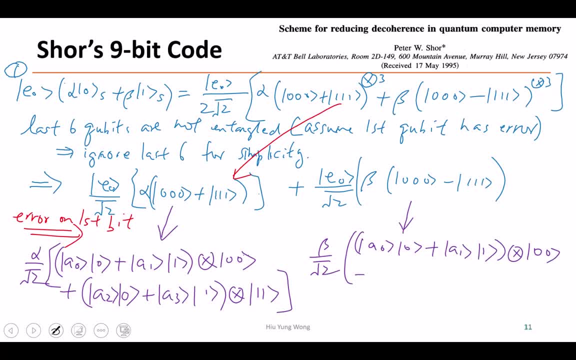 tensor product: zero, zero, minus. what is the second one? A two, zero plus A three, one. very good, this is the first qubit tensor product of one one. everyone can follow any question, just ask. right up to now, you see, this is pretty nice, actually, the zero and one they are. 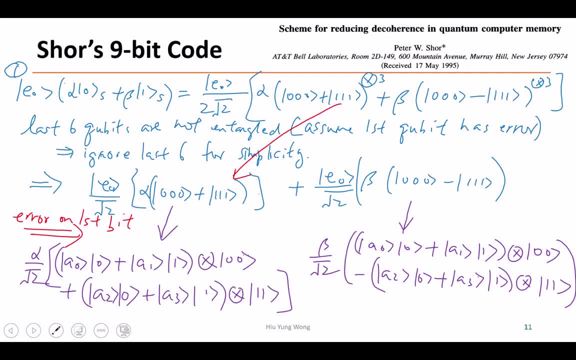 repeating each other. that means later. you can factorize that. why is that now? I will continue to do this, but if I do this, I think it will be difficult for you to see, but I will still do it. what I am going to do now is multiply. 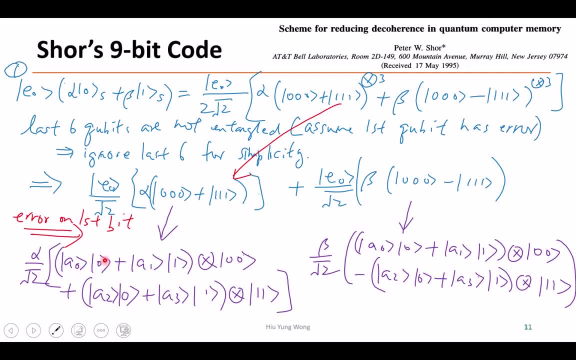 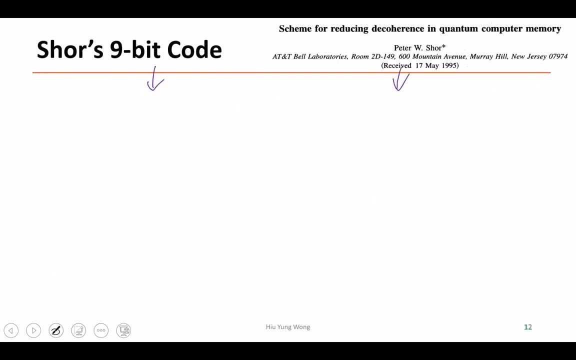 A zero. this is zero, zero, zero. this is one, one, one right. so I have A zero times zero, zero, zero, and then what I am going to do is to split it so that I have this- I know it is from the last page, right from the last page. 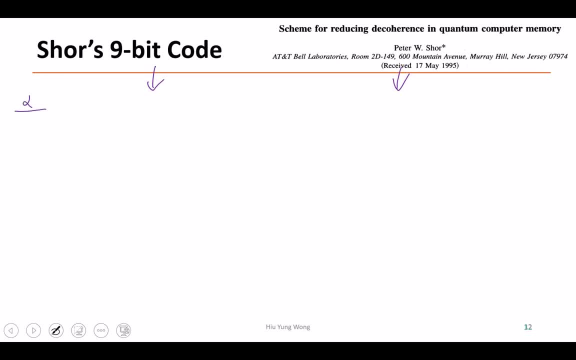 let me write it down first. I can change what I had from the last line to be this: A zero plus A three right times zero, zero, zero plus one one one, and then the whole thing: plus A zero minus A three times zero, zero, zero minus one one one. 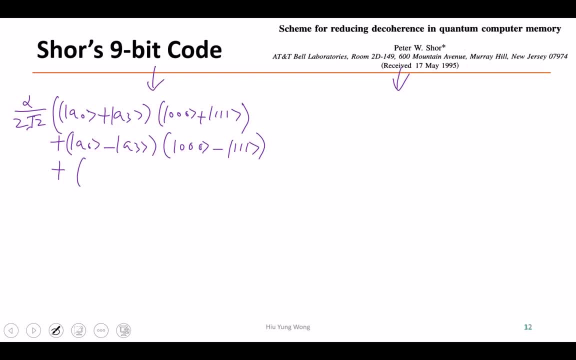 right, I don't think you need to be able to follow now. I will just show you what happened, and this is just math. you can do it easy to show that this is correct. let me finish writing. sorry for that very long. right, I know it is very long. 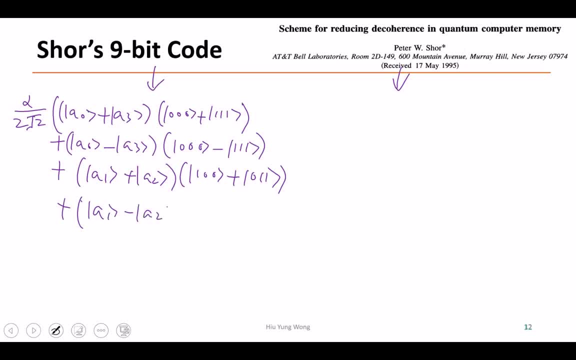 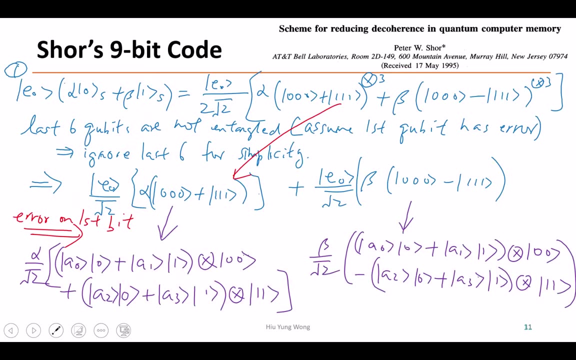 but you need to see it at least one time in your life- one zero, zero. and you need to understand why they came up. they were able to came up with this right. I claim that this whole term equals to this one. okay, let's see if that is the case, for example, how many. 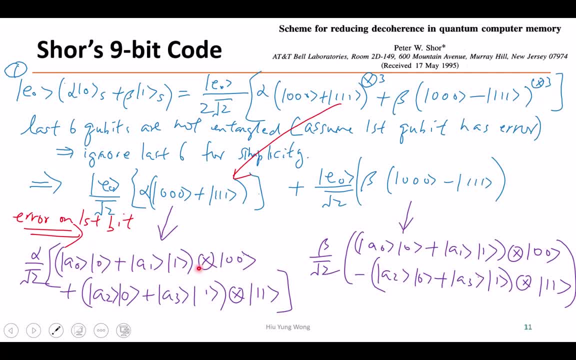 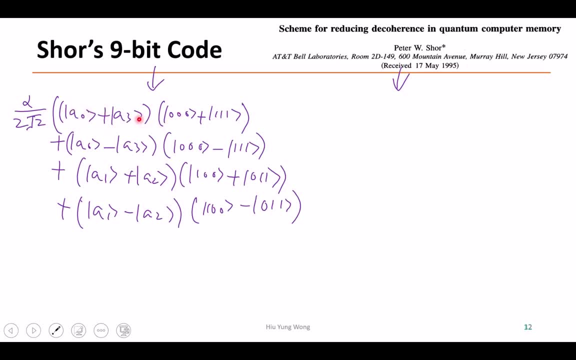 zero zero do I have? I only have A zero, zero, zero, zero, right. but here, how many zero zero do I have? I have A zero plus A three zero, zero, zero, A zero minus A three zero, zero, zero, right. but this is negative, this is positive, right. so they are going to get cancelled. so I have 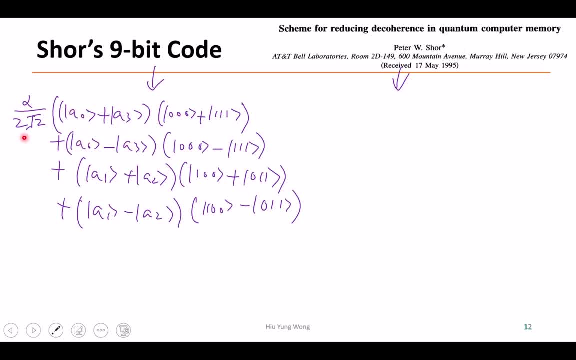 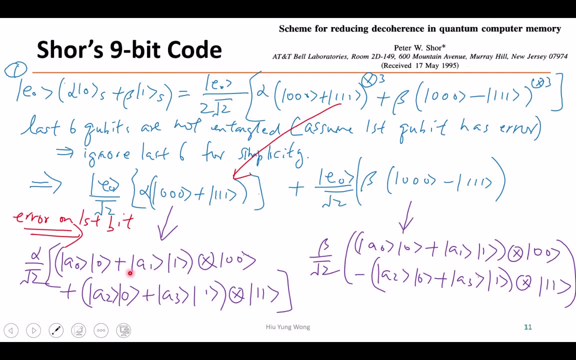 two A zero, zero, zero, zero. but I divide it by two, so if you expand it, you only get one zero, zero, zero. that is what we have here: one zero, zero, zero. how many one zero zero we have? we only have one A one zero, zero, right, if you look at? 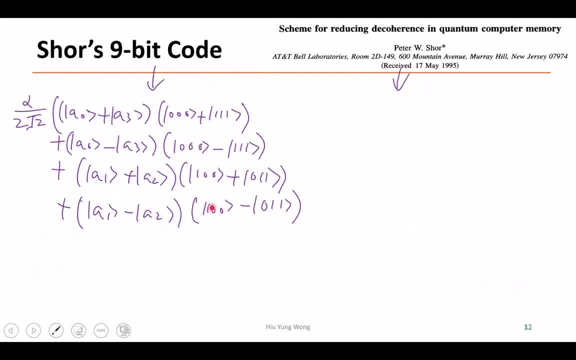 this how many one zero zero we have. I have two, but then I have A one plus A two, A one minus A two. so when you add them together, I only have two A one, one zero zero divided by two. again, it is correct. yeah, yeah, no error is on the MSB. 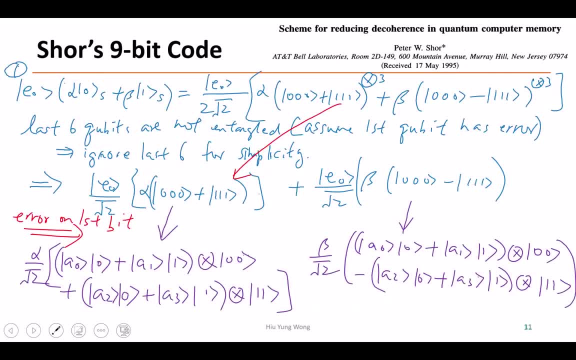 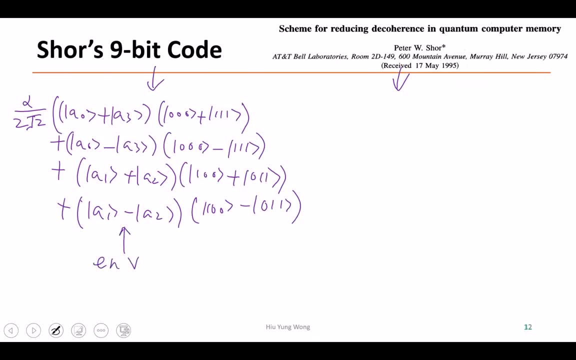 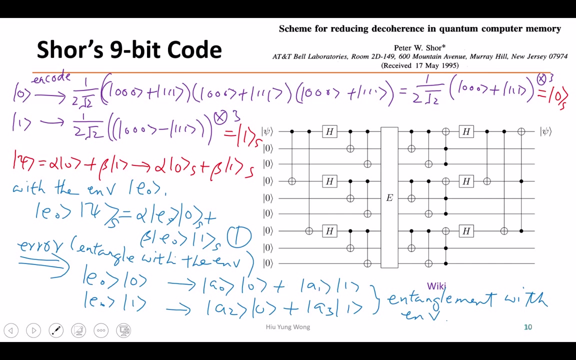 yeah, error is the MSB right, so these are the error, right. say again: let's don't call it error, let's call it the environment state, okay and yes, and. but when you entangle with your qubit, it becomes an error of your qubit. yeah, 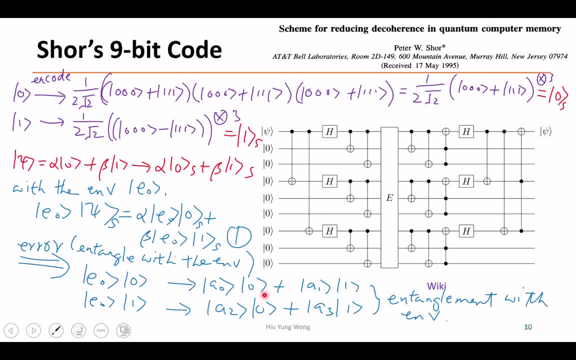 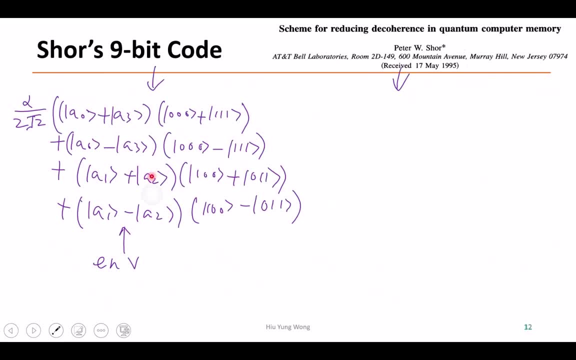 so originally I have very pure zero. now it becomes something zero plus something one, right, I don't know whether it's zero or one, but but the point is that now I do, by using this nine qubit code, I come up with this: three states. but what is the correct state? the 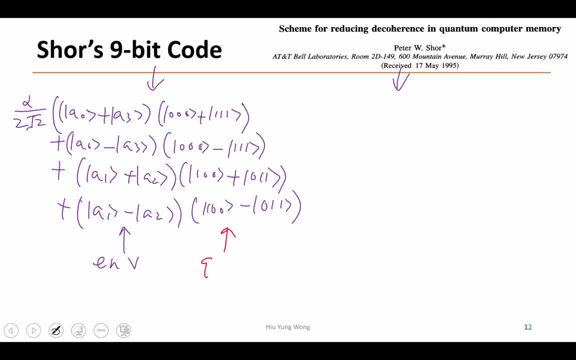 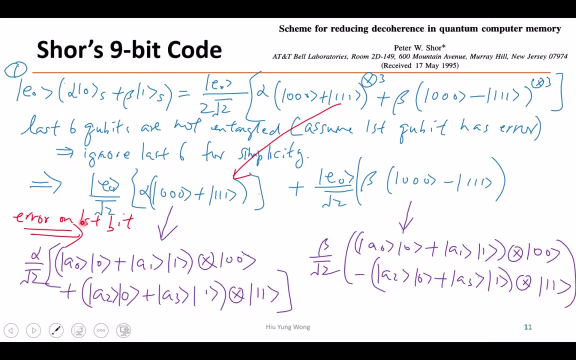 correct one is what? this is the qubit right that we want, right, the three qubit the correct one supposed to be? what for alpha? what is the correct one supposed to be? let's look at before we apply the error. what is the correct one? zero, zero, zero plus one. 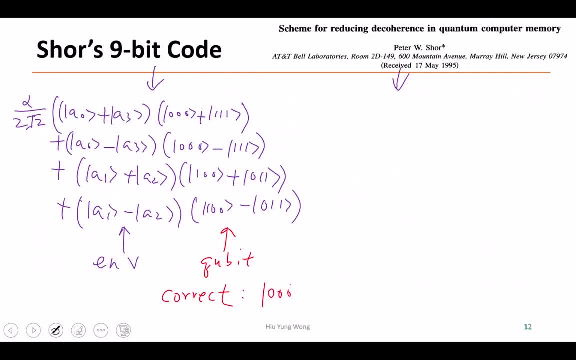 one one, zero, zero, zero, plus one one one. okay, of course, the last nine qubit are the same. without talking about it, now let's take a look on the beta part. on the one part, the beta part, which was the original one of this qubit, what is? 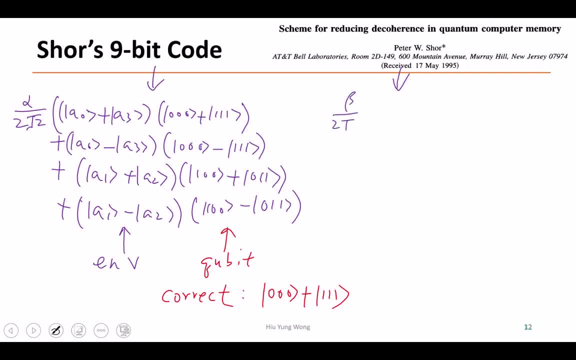 that let me also copy it beta over two square root two. again, you don't need to copy because next page I have the whole equation right. but I want you to appreciate the what is so good now, because now you have try to see what is the. what are the comments between? 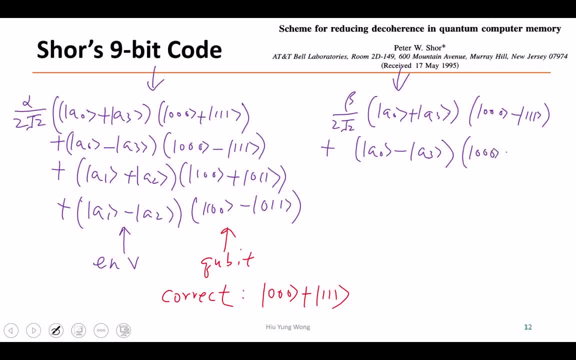 the one and zero, or the beta and alpha. so one of the terms for these- from the beta survives beta, one, one, one- is that what you're getting at, what you get is: do you see that they have the same environment in front of them? well, but these are not the same. 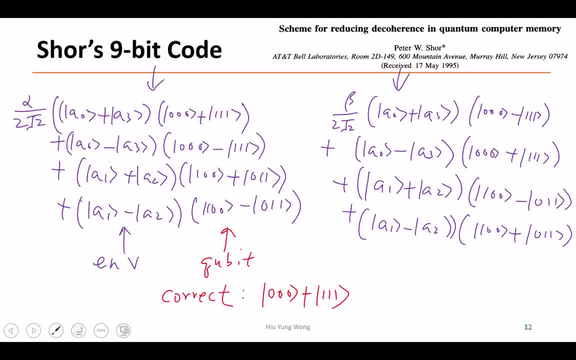 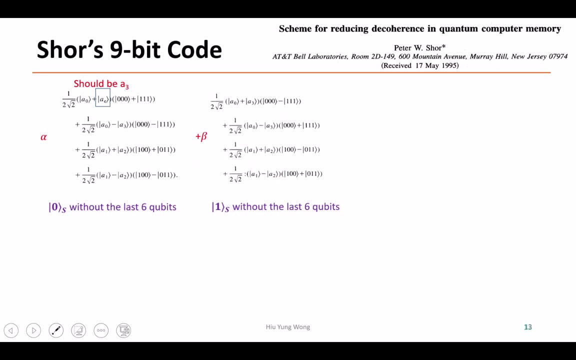 however. yeah, but they have the same environment now. so then that is how you do the correction, right. so here I show you the final results again. that's why you don't need to correct here. we don't have the last six qubit, but the last six qubit are the same for. 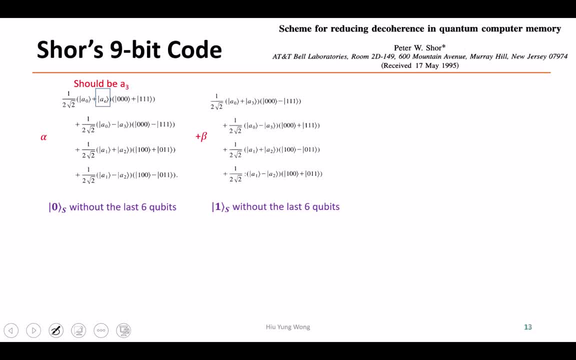 all of them. okay, so that is what we do, so we will measure. we did not show here right, did not show. yes, this is only the first three, because we only have three qubit here, right and then. but the last qubit is just zero, zero, zero. 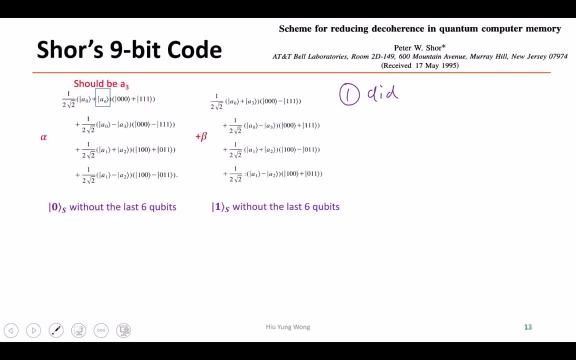 plus one, one one, the last six, one, two of them. yeah, so you are going to have zero, zero, zero plus one, one one, zero, zero plus one one one for each of this superposition, right? so we, what we will do is to create an entanglement. 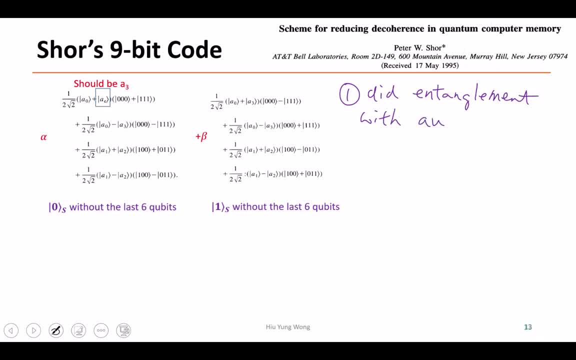 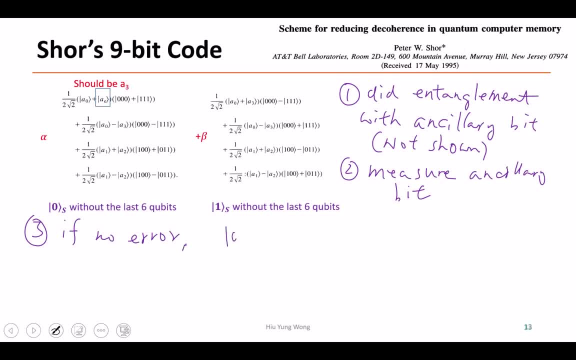 be what we expect it to be: 0 0 0 plus 1, 1, 1. alpha plus beta. 0, 0 0 minus 1, 1 1. correct, because this one is the encoding for 0. this is the encoding for 1. I did. 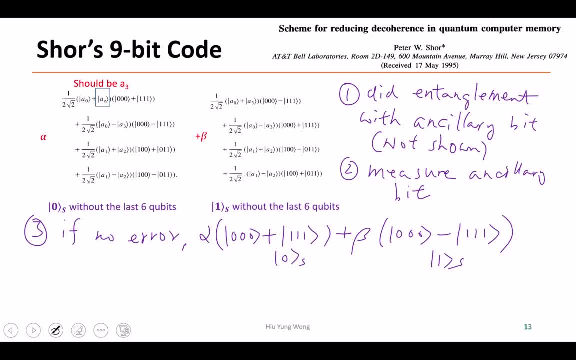 not show the other 6 qubit correct, if there's no error. so if we do the correct encoding of this, we do an entanglement of this qubit with an auxiliary bit. we measure the auxiliary bit, we find that all that is correspond correspond to this. then you do nothing, you. 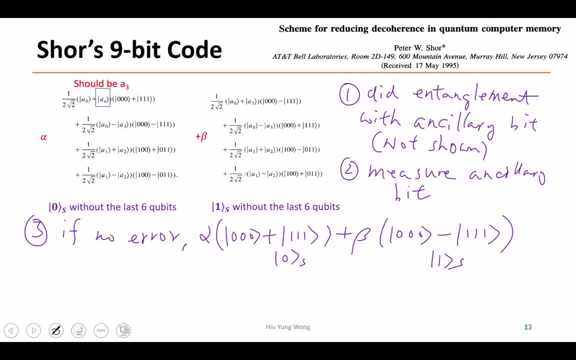 just apply an identity gate right now if, for example, you got a, let's say, the second row with second row I mean. what I mean is if the auxiliary bits- the auxiliary bit is not shown in this circuit, but we will do some entanglement with this- we we can always entangle the state with the. 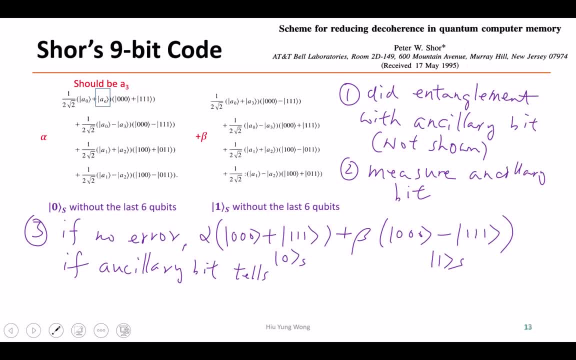 auxiliary bit. okay, and then we measure the auxiliary bits based on the value of the auxiliary bit. I will know that, whether it is this state or this state, yeah, so you're calling ancillary bit is what's Ancillary? sorry, not auxiliary. so that's the error syndrome, right? 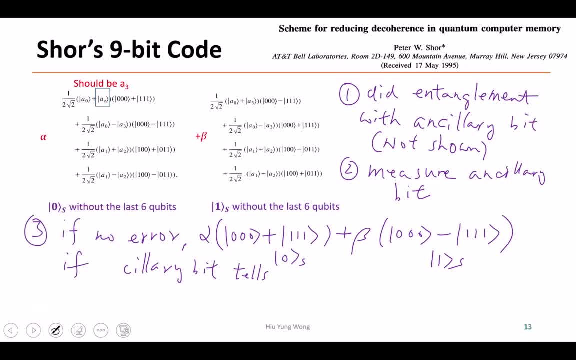 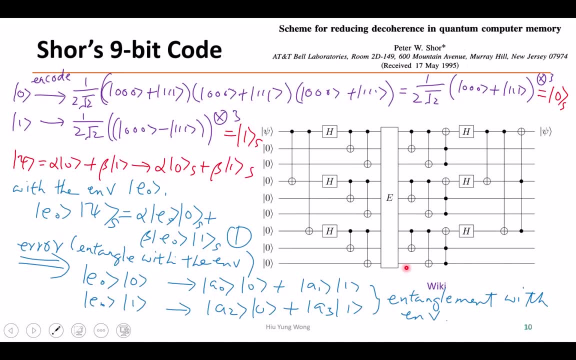 yeah, there is a syndrome, but can you maybe point where are you in the circuit? when not in the circuit, why circuit? we did not show them. no, this one doesn't have the ancillary bit, so so because this one, come up with some auto correction. so in a real case you. 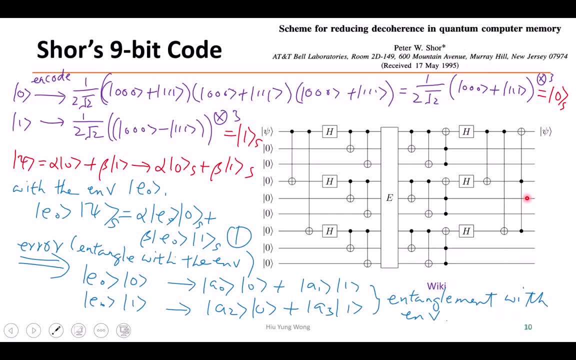 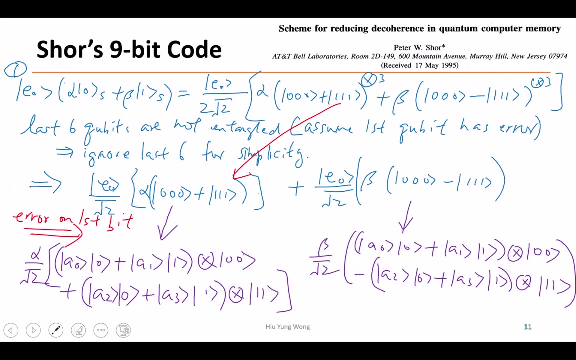 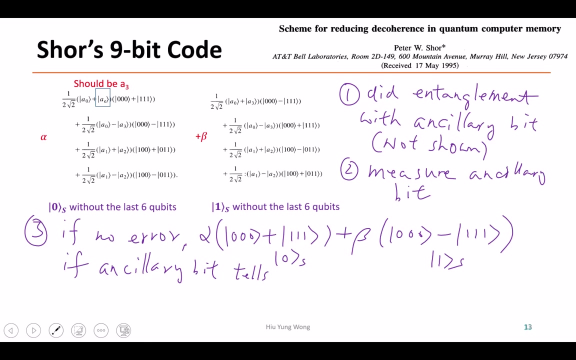 actually need to go to the ancillary. you do measurement and then you apply. okay, here is no ancillary bit, this one is just based on the result, automatically correct. okay, this is not the original Shor's circuit. okay, just that it is not shown here. you need to do the measurement, your measurement. 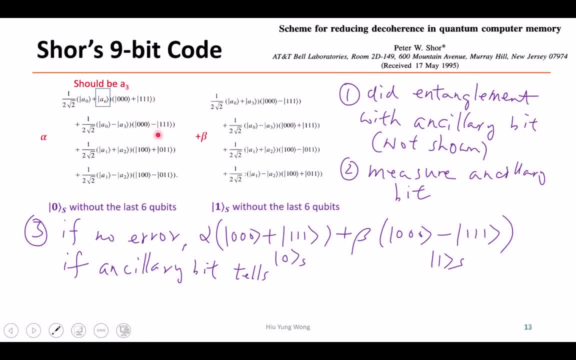 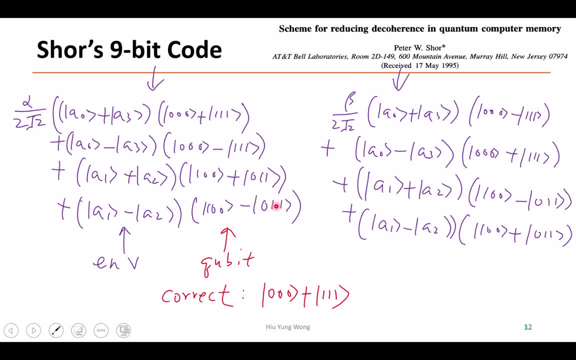 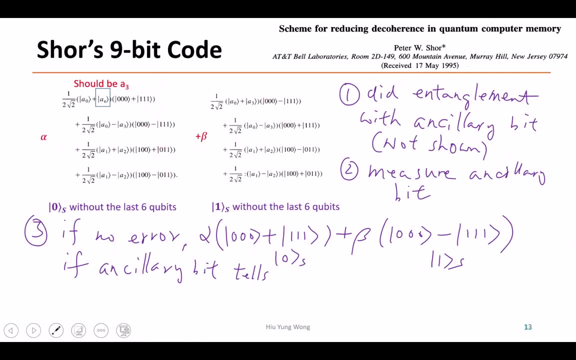 will indicate whether you, whether you are, in which state you were in here, what type of flipping you have. so you can see that from this whole exercise it gives you a general error, but this general error eventually decomposed to this four type of possible output. these are the 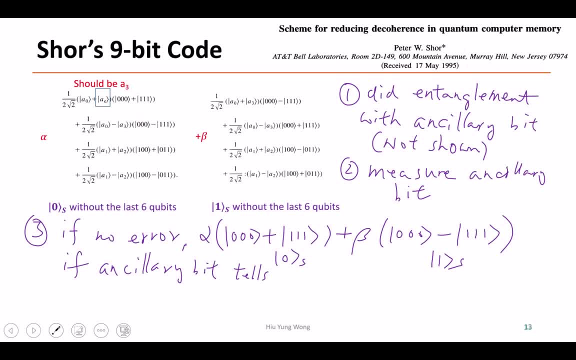 Bell state. okay. and then, because if you entangle this Bell states with ancillary bit, you're, by measuring the ancillary bit, you know that which state it becomes, and then you apply the appropriate correction. you know that which state it becomes, and then you apply the appropriate correction. 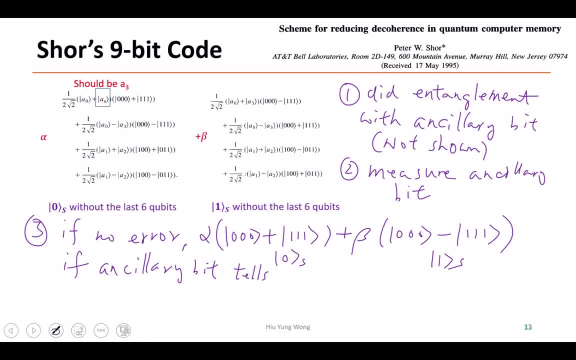 so if the ancillary bit tells you that it is, for example, there is a wrong side, for example the second row, right then you know that. okay, my second. actually, what I have is this second row. so what should I apply in order to get back what I want? so this, I am supposed to get this and this right, but now this is got this. 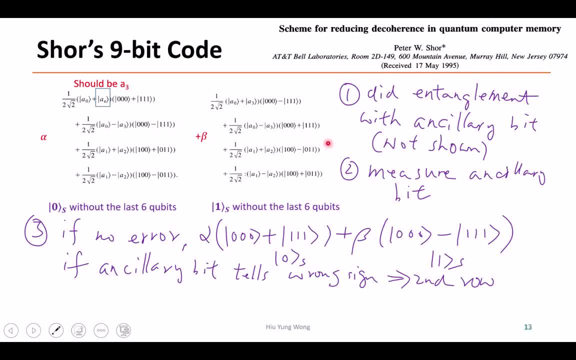 is. you can see this is the second row and then you apply the appropriate correction. you can see that this is a what sign flip. this is a phase shift, right? so you apply z gate. right, you apply a z gate, then you can bring it back to the. 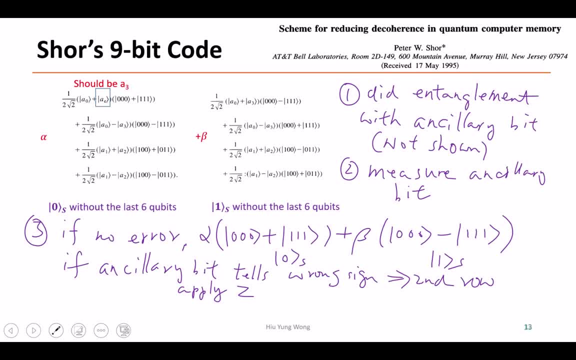 correct answer. okay, so I only show you how it work. I don't have insights for you how they came up with this, but the most important thing is you see that if it was done such a way that the zero and one encoded zero and one have shared the same environment value, that's why you can factorize it out- if 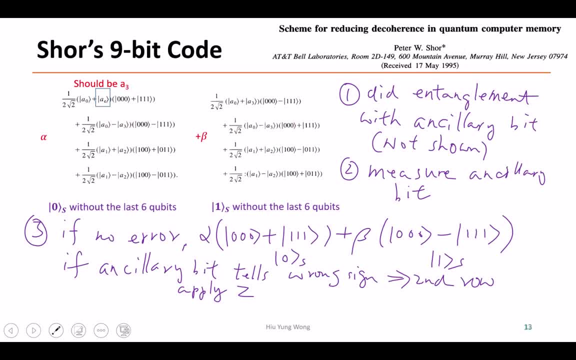 they don't share the same value. you cannot factorize it out right when. yeah. so let's say, if the environment for the MSB is different from the LSB, then this regime doesn't work. you cannot, because I already proved a general case. these are the only four. 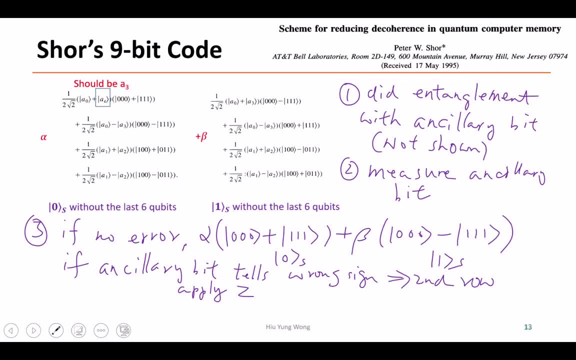 possible value. yeah, this, a zero minus a three. a zero minus a three. this is the environment qubit state right. it's a superposition of two states of the environment that they have the same right. so when I add them together I can factorize it and then my qubit still in this state right.